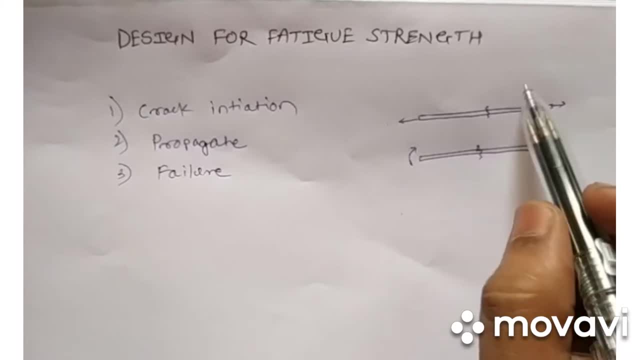 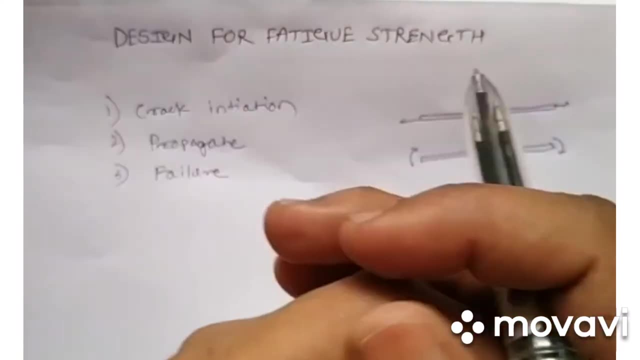 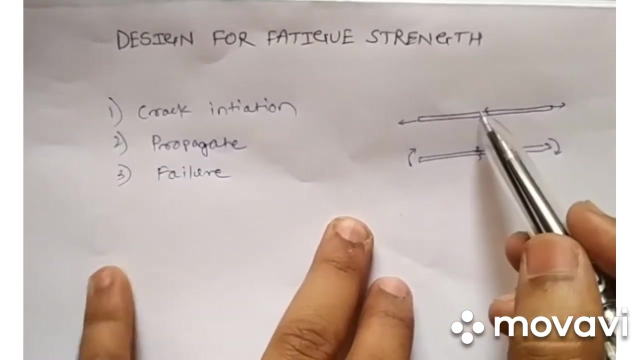 and try to break this wire, it will take much strength. but instead of that, if I try to twist the wire like this, which we do generally, to break the parts, so we can observe that this wire will get failed much earlier as compared to this example number one. okay, this will fail earlier. 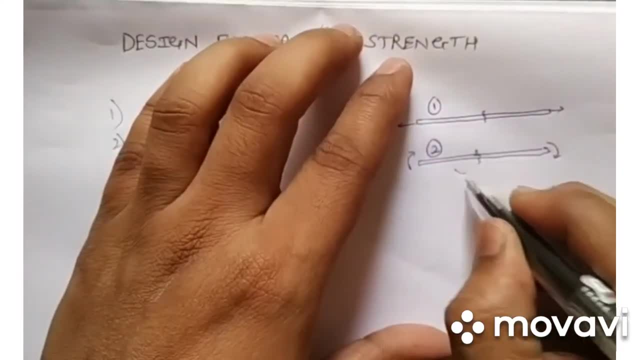 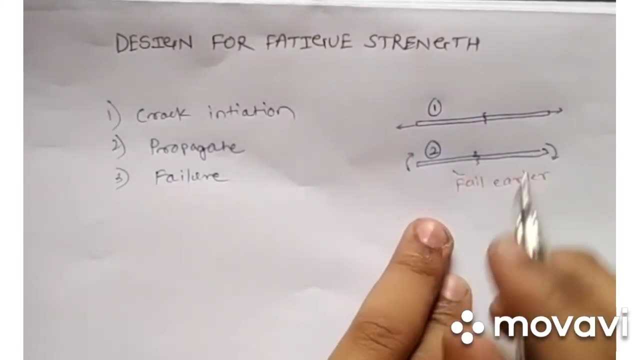 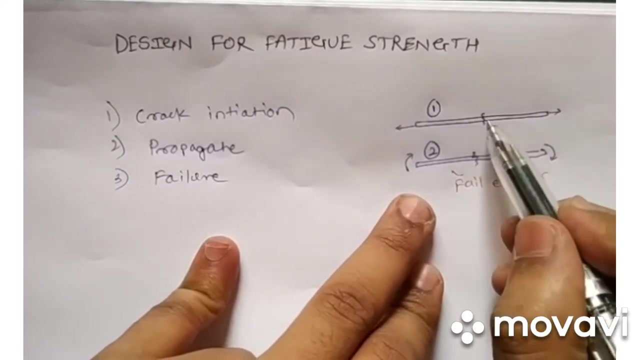 as compared to one. okay, earlier. okay, and it will fail earlier because it will fail to a stress value lesser than the static strength of the- let's consider it's a steel. then it will fail to a value which is lesser than the static strength of the steel. so this is nothing but. 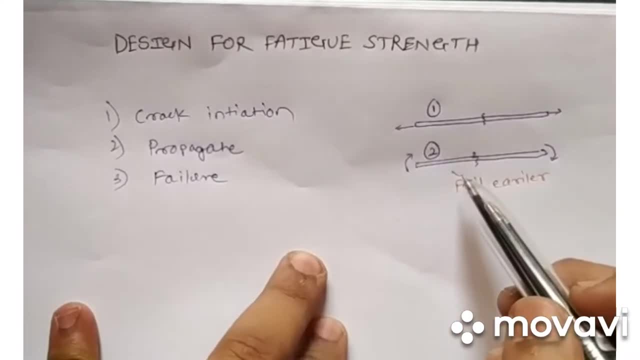 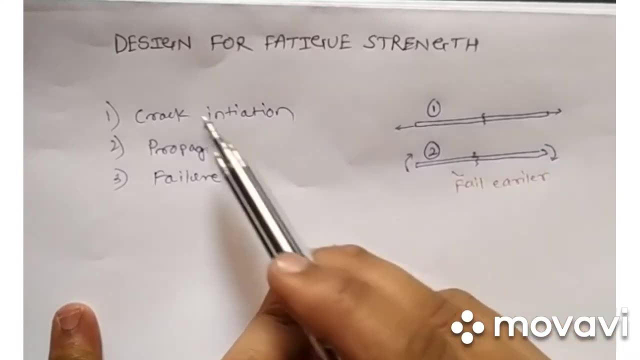 failure because of the fatigue which is getting induced in the body and because of that the material is getting failed. okay, so how it fails? when there is initially crack initiation in the body, then this crack gets propagated through the body and finally the material fails. okay, now there. 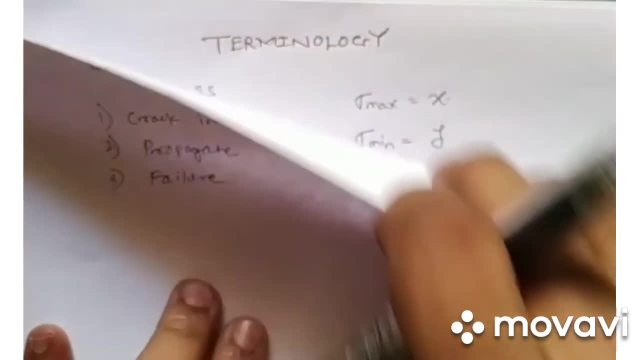 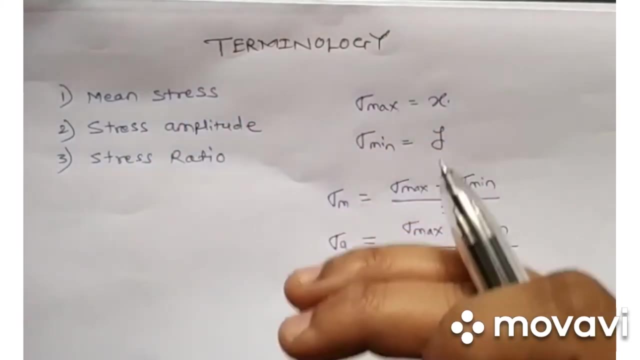 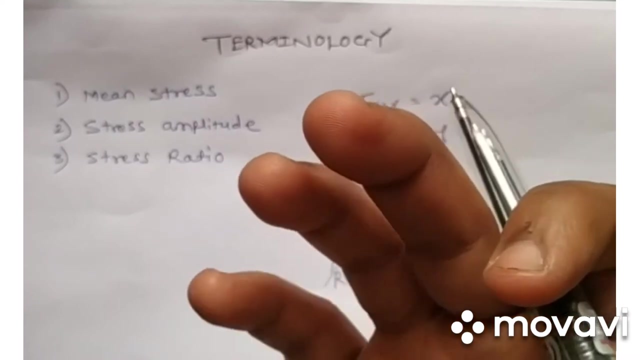 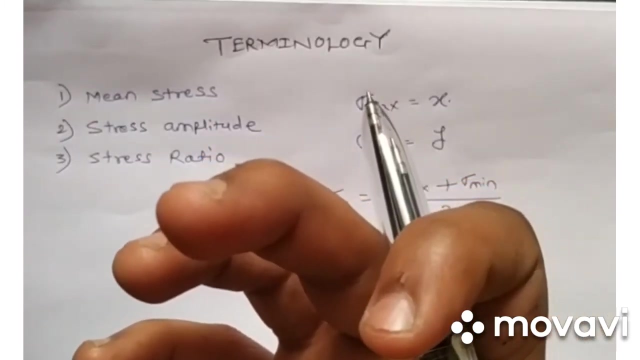 is a very important to know. so we will get into those terminology. so first is mean stress. okay, now when I say fluctuating stress, the stress values and magnitude can be changing. okay, when I say 40, let's consider if a body is subjected to tensile load. now the direction of the loading is. 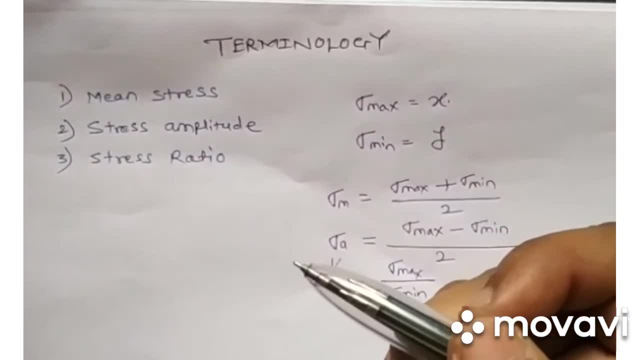 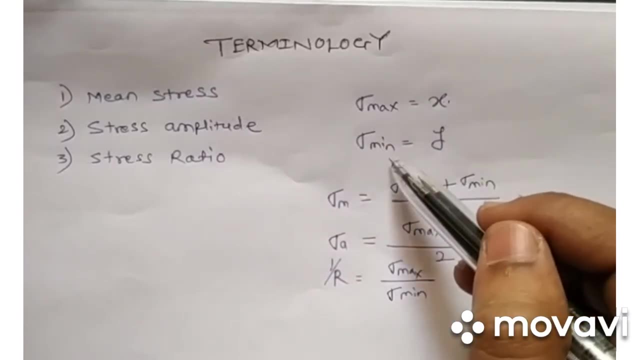 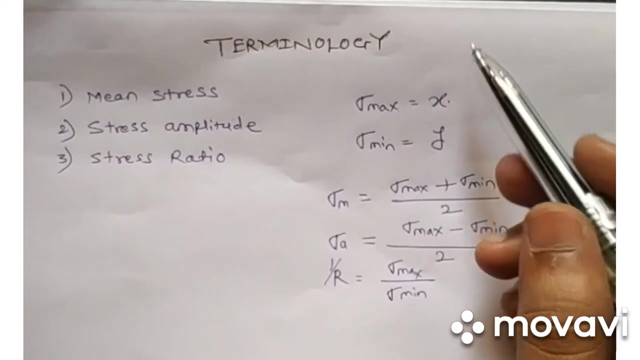 same. that is tensile, but over the period of time the value is getting changed, so it has some maximum stress and it might may have some minimum tensile stress. likewise, if a body is subjected to come compressive stresses, so it will have some maximum value of stress over the period of time and might have some minimum value of compressive. 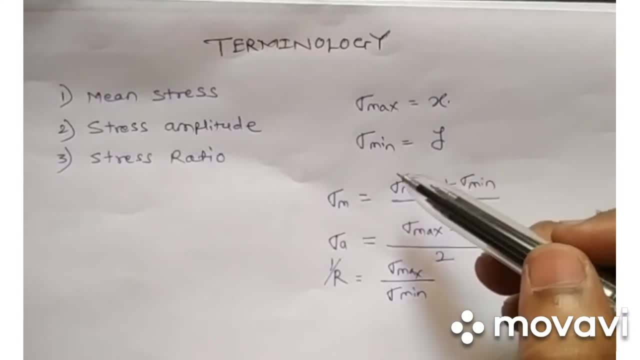 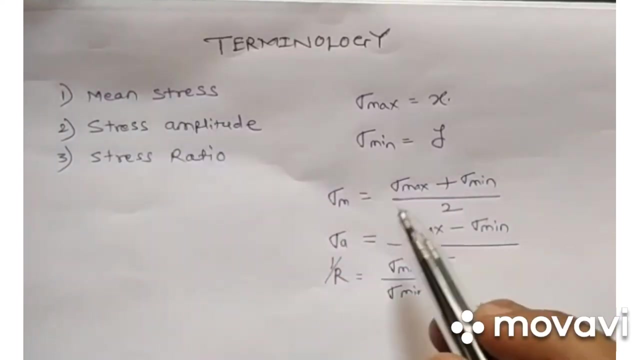 stress over the period of time, or the body can be subjected to completely reverse loading. so we will going to see those things first. consider this terminology. okay, so the body will be subjected to some maximum value and some minimum value. now, first, is Sigma mean stress, which is denoted by Sigma M, and it is nothing but the. 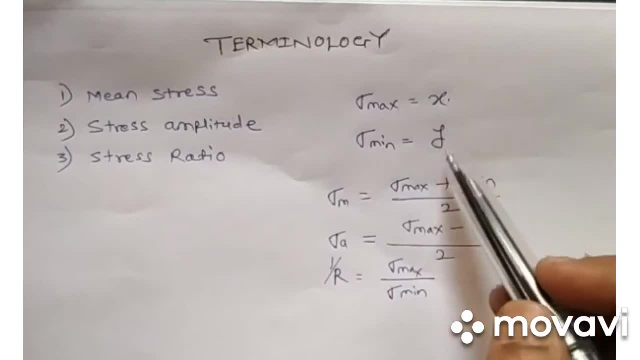 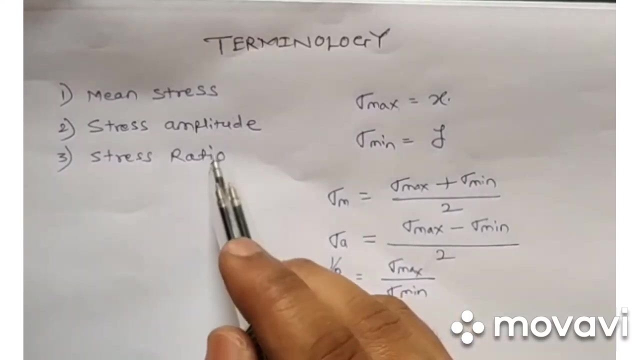 mean. it is a basic thing. so it will be the mean of this maximum stress and the minimum stress. then we have a stress amplitude, so it is nothing but Sigma maximum minus Sigma minimum by two. and then we have the stress ratio which is denoted by R. so one by r is Sigma maximum by a minimum. so we can. 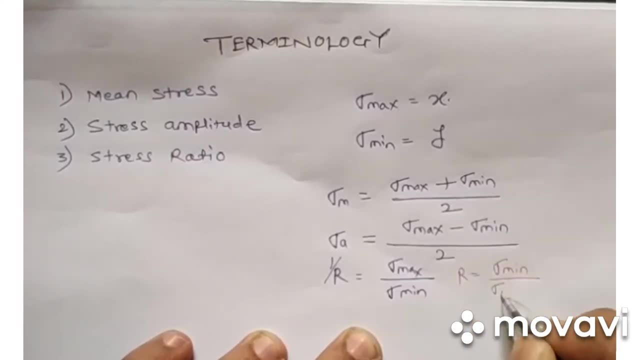 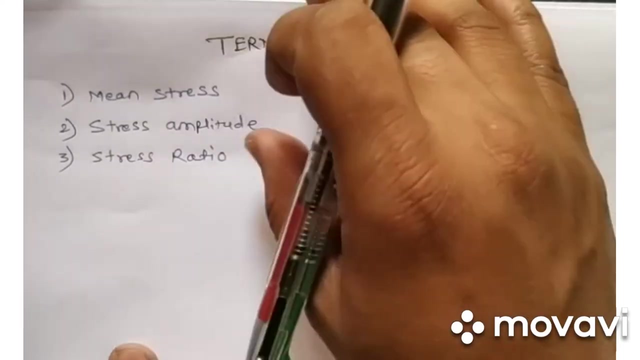 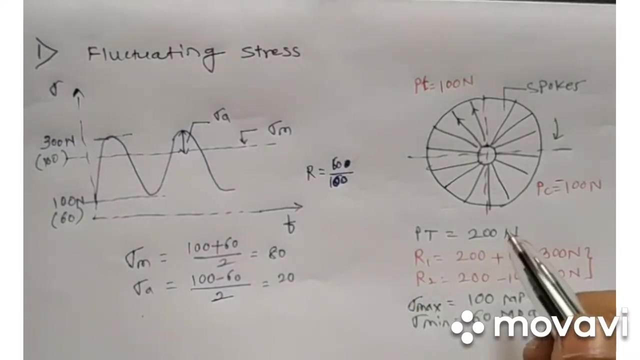 write R as Sigma minimum by Sigma maximum. so this is nothing but stress ratio. so this terminology is very important to consider the different types of loading. now. first let us consider the fluctuating charge, Bay stress. now we can understand this concept with the example. so this is a bicycle wheel and these 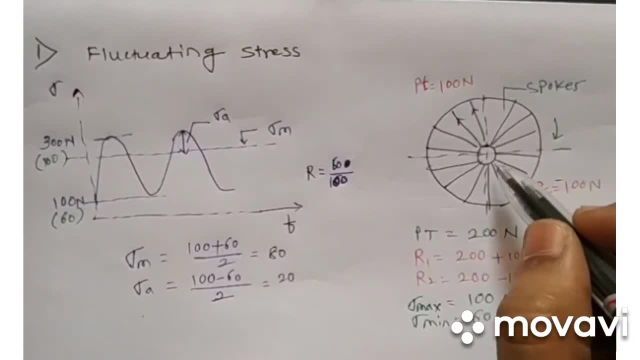 are the spokes attached to the hub. okay, now these spokes are pre-tensioned. that means there is initial tensioning of these spokes. now why it is required? now we know that when the bicycle run, the spokes come under the compressive loading, then the tensile loading, compressive loading. 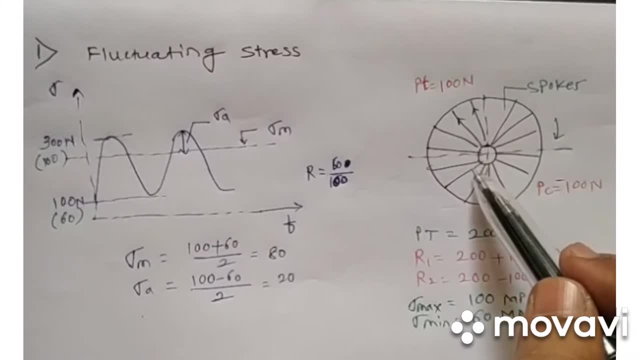 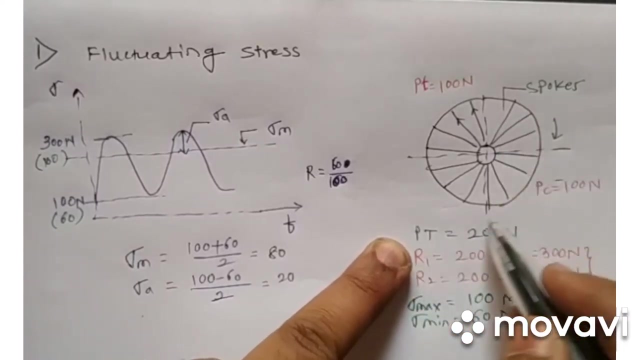 tensile loading. so the spoke has to take both compressive and tensile forces. but the wire is not able to take the compressive stresses. so what we can do? so that the resultant load coming on the wire should be tensile, and so the stresses are tensile. so for that purpose these wires are pre-tensioned. now let us consider these wires. 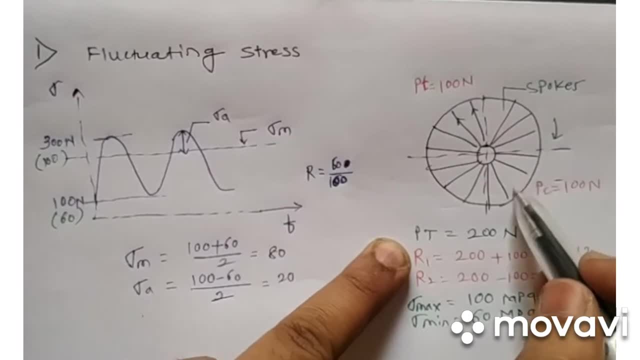 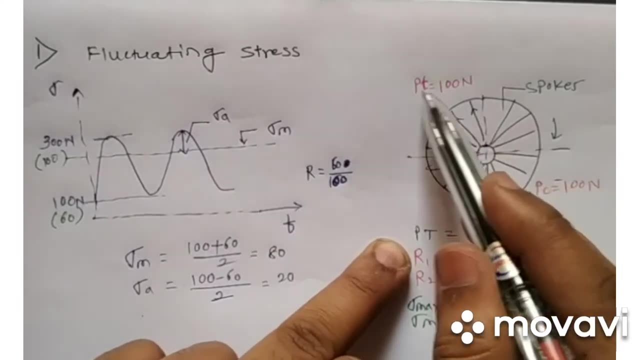 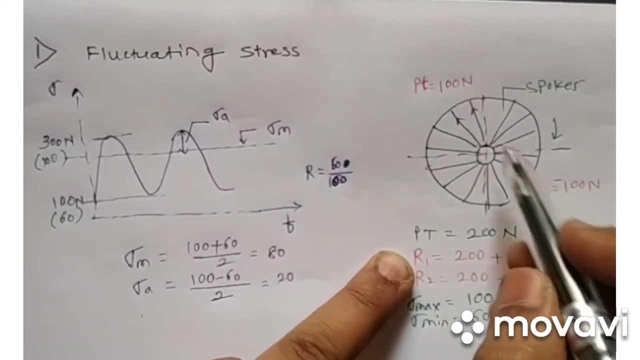 are pre-tensioned with 200 newton. now, when these spokes come to this position, let's consider- they are subjected to compressive load of 100 newton. when they go to top position, they are subjected to tensile loading of 100 newton. now, if you see the resultant load, now for this condition, the 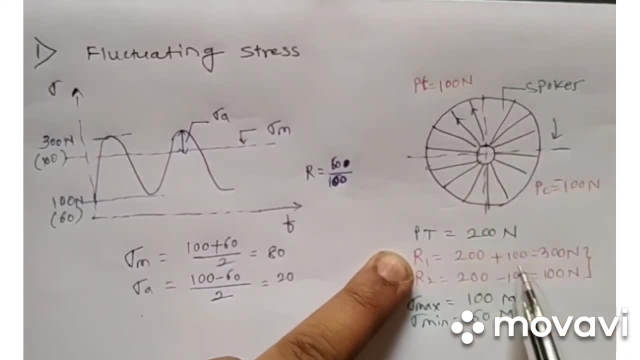 resultant load will be the initial pre-tension of 200 newton newton plus the tensile load of 100 newton, so the resultant will be 300 newton. likewise, when these spokes come to this position, they will be under compressive load, so the resultant load 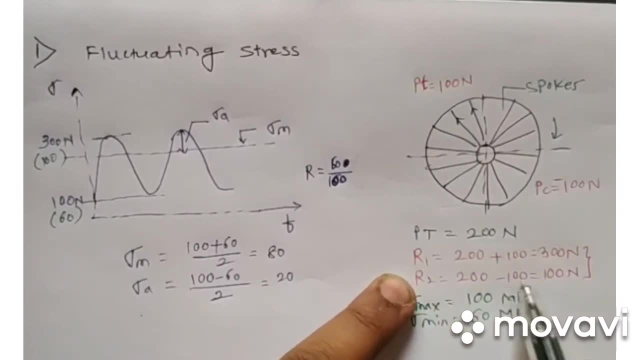 will be 200 minus 100 minus, because it is compressive. so the resultant load is 100 newton. now here you have to focus. we have achieved our target. that means we wanted that spokes should be under tensile loading also, and here we have achieved it. so this is the importance of 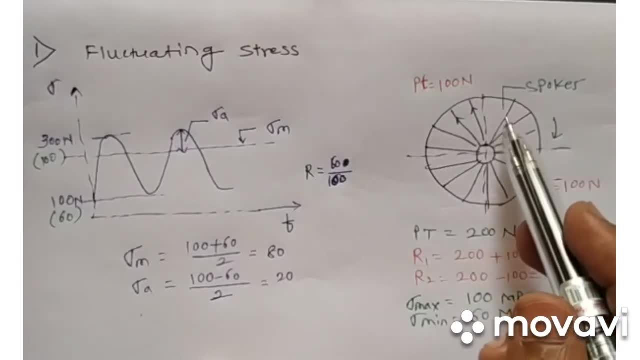 pre-tensioning. now, with considering the cross section of the spokes, the spokes will be subjected to some maximum value of stress, which is corresponding to this maximum value of load, and some minimum value of stress which is subjected to this minimum value of load. so we draw a graph which is: 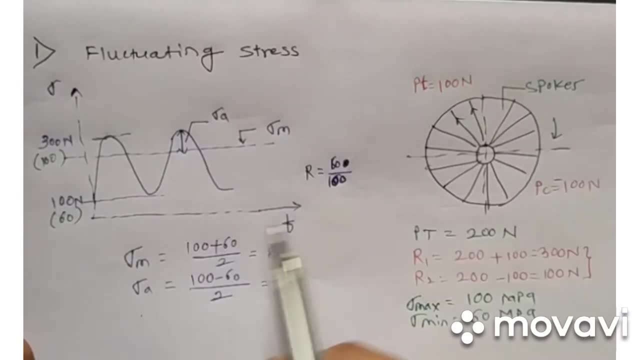 you sigma against t, that is the over the period of time. so this is the maximum value of stress, and this is the minimum value of stress. we have plotted the graph, so we have found out the sigma mean and sigma amplitude. now, in this case, sigma mean will be 100 plus 60 by 2, that is 80. 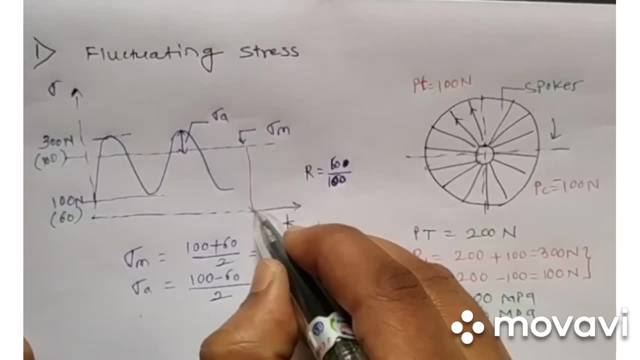 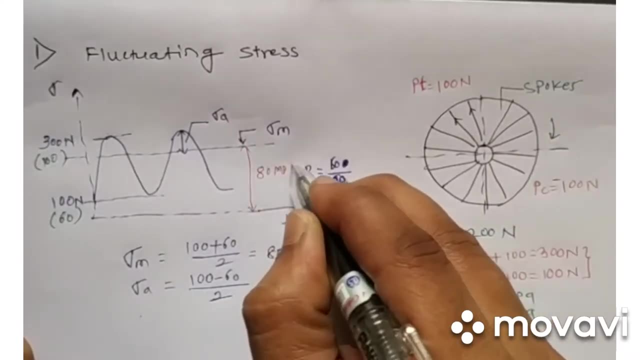 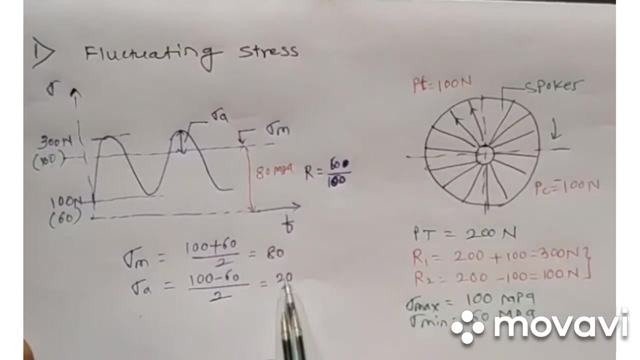 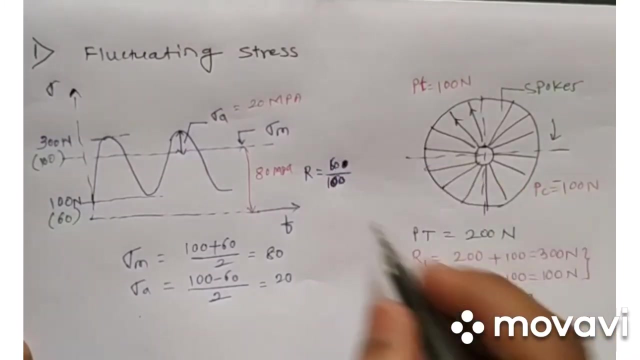 so this value is nothing but your sigma mean, that is 80 mpa. let's say, and sigma amplitude is 100, maximum minus minimum by 2, that is 20. so this amplitude will be 20 mpa. and now the r value. so minimum value is 60 and maximum value is 100. so this value 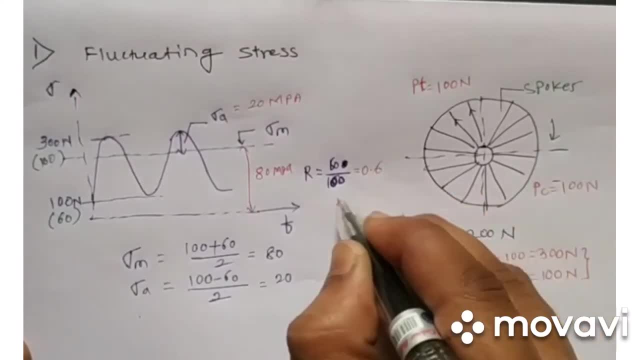 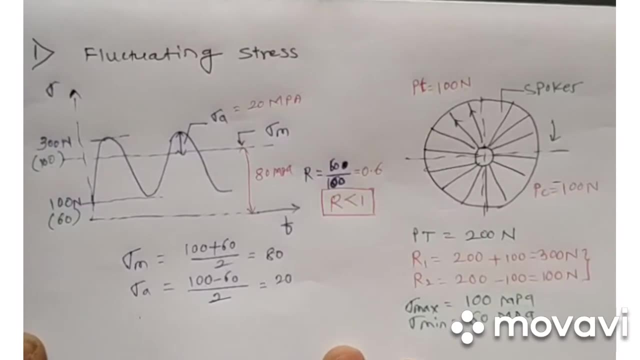 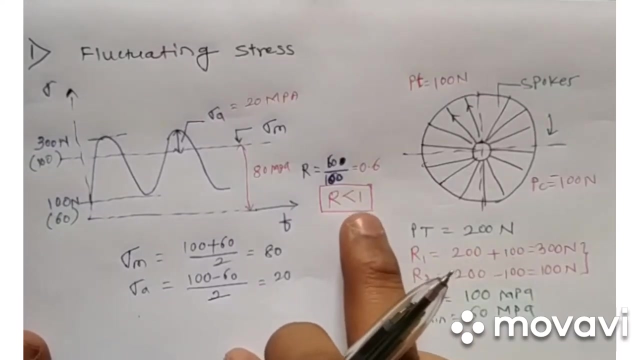 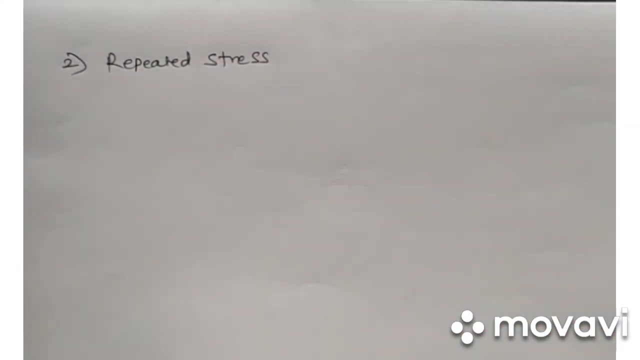 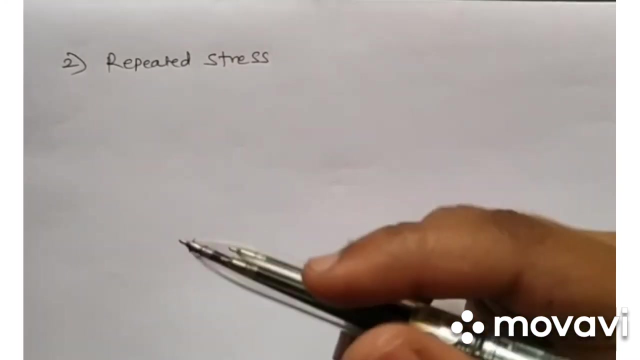 will be 0.6. so in this case the r is lesser than 1. okay, so for fluctuating condition, this r value is always less than 1. now let's get into other type now: repeated stress. now, the name itself indicates repeated. that means the body is subjected to a. 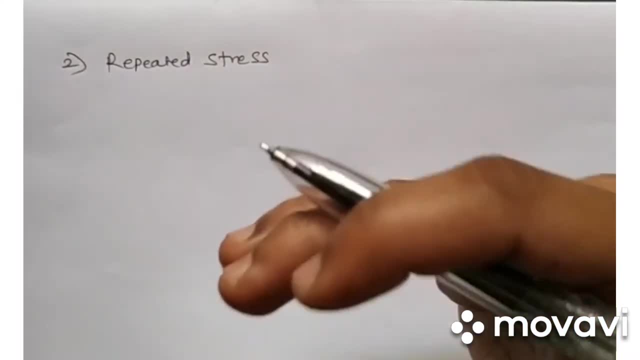 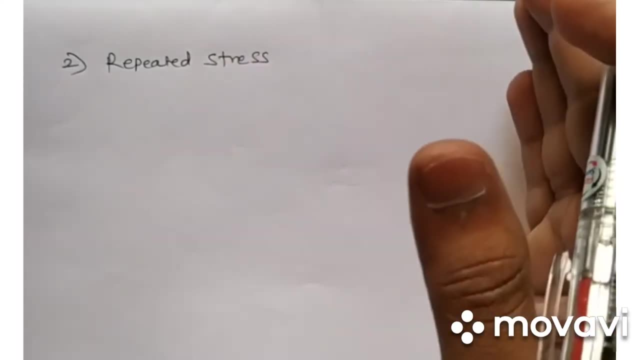 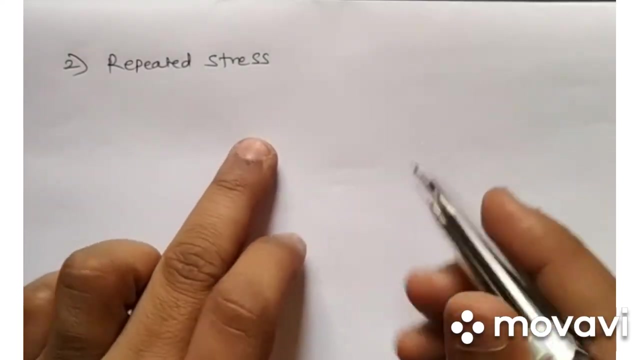 repeated type of stress. so this is the repeated type of stress. so this is the repeated type of stress. but here the stress value, that is, the magnitude, is getting changed, but the direction is same. so this is main thing you have to understand: repeated. so let's consider example: uh, let's consider a 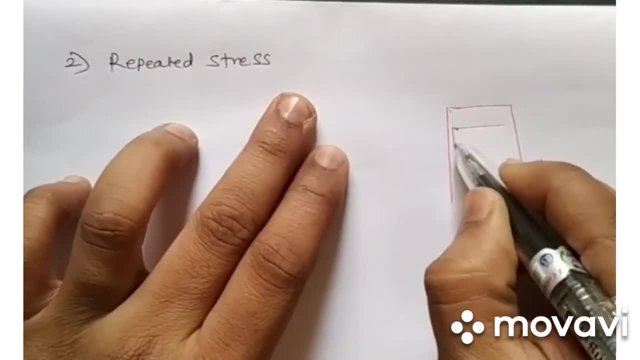 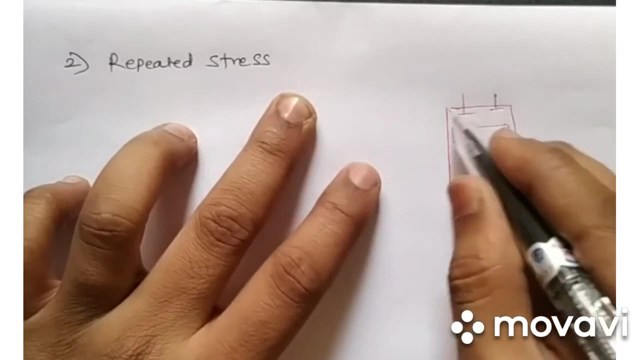 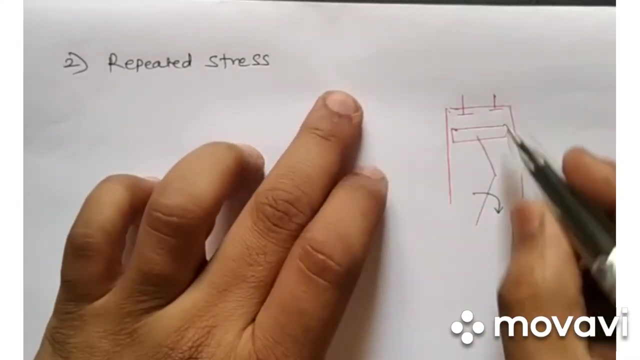 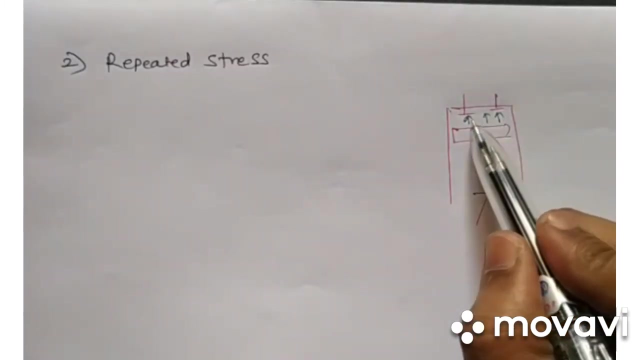 ic engine. okay, there is a piston and connecting rod, all those things. here there are walls, okay, and this crank rotates and we know that the gases exerts pressure on these walls. okay, now they will exert the pressure on these walls, so compressive stresses will be generated here. okay, and we know the cycle of the ic engine, so at each cycle there is one. 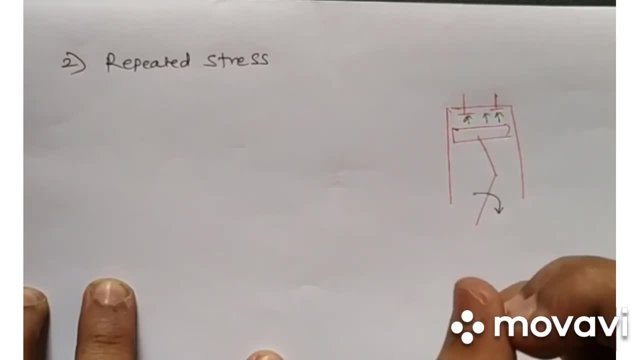 power stroke and at that power stroke the gases burns and, uh, you know, they just exert the pressure and because of that, these walls are under the stresses. so this is the case of the repeated condition. okay, so let's try to have the graph for this condition, um, okay. 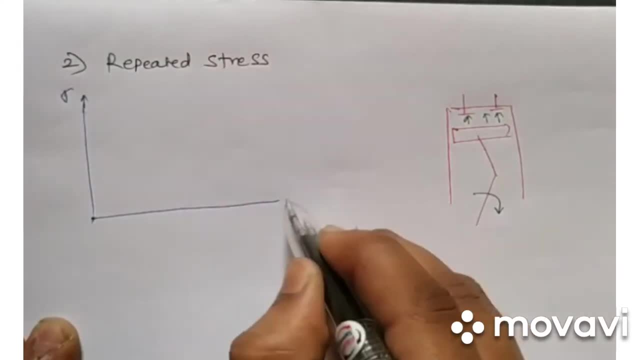 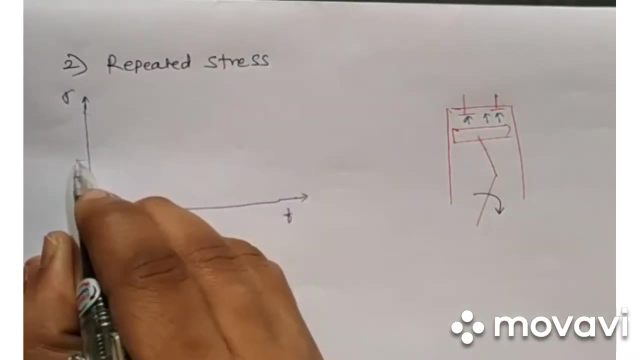 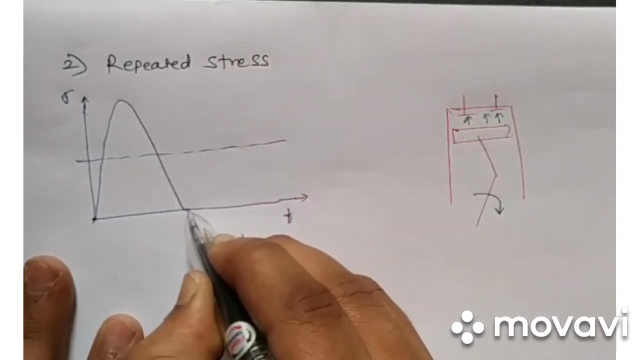 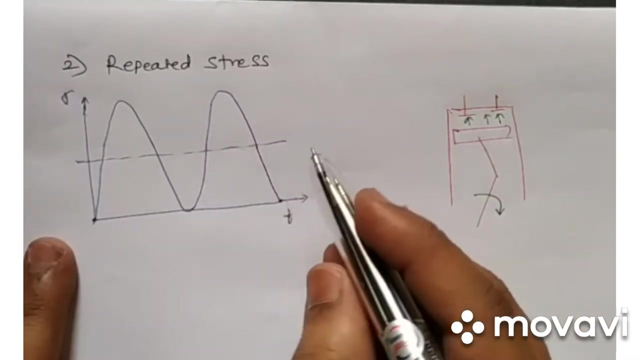 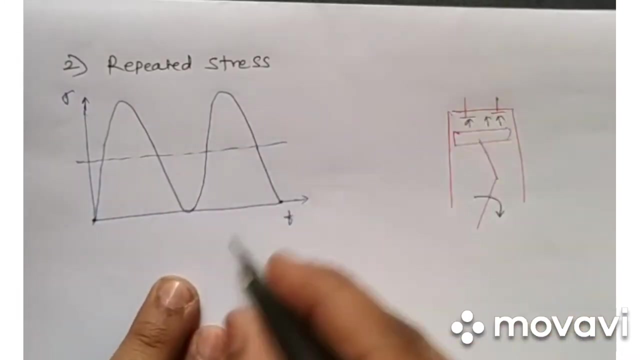 so here we have a sigma, here we have a time and repeated so the value it's, you know, tensile, it is varying on only one direction and let's consider subject, of course, subject, of course, one direction to. we are taking just an example. so Sigma, now this is the repeated stress. 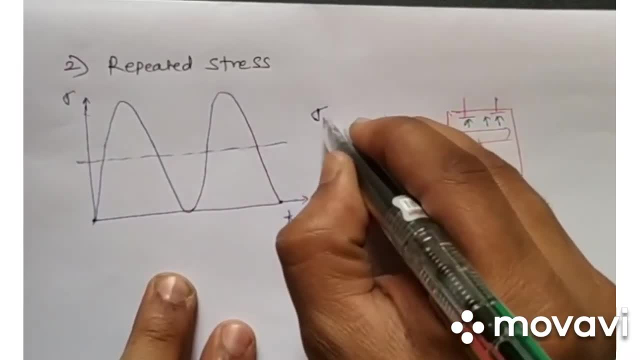 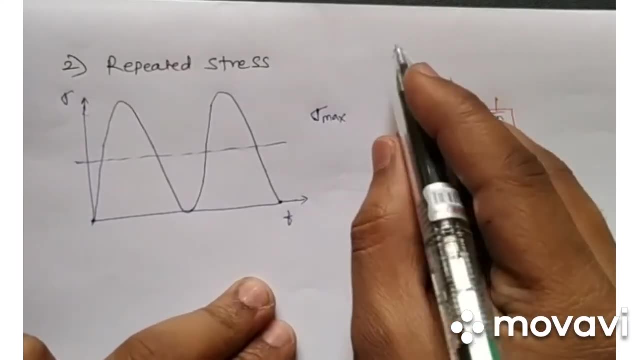 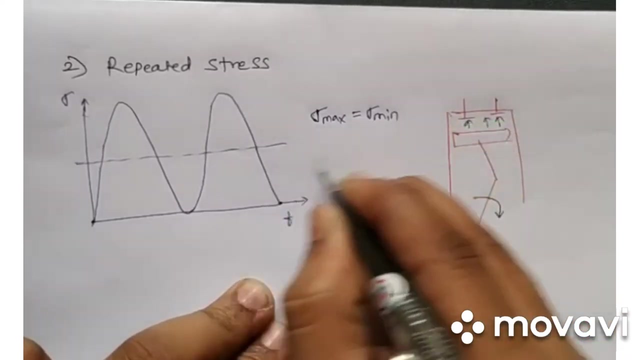 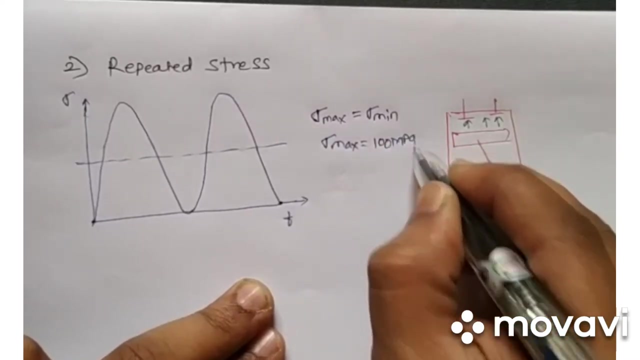 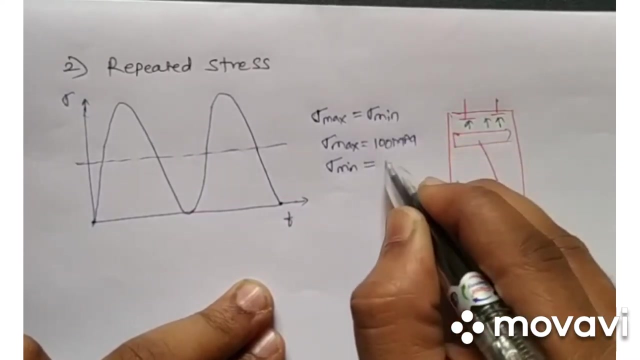 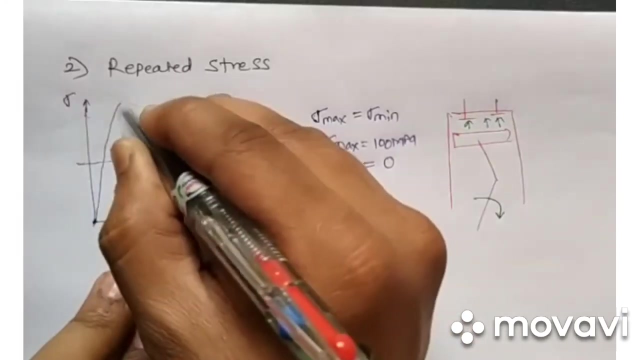 the magnitude is same. so what we can say here: Sigma max is equal to Sigma minimum. okay, because it is repeated. so let's say Sigma max is 100 MPa and Sigma minimum will be 0. okay, that means it is subjected from 0 to some higher value. 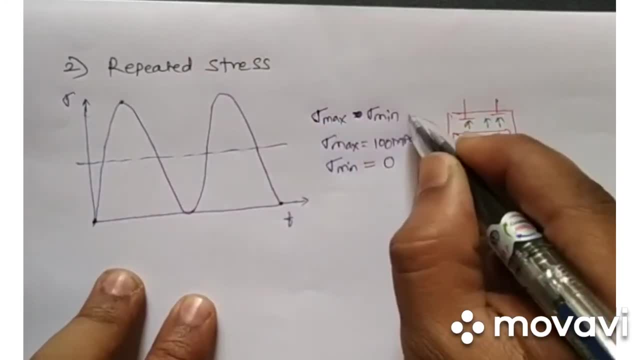 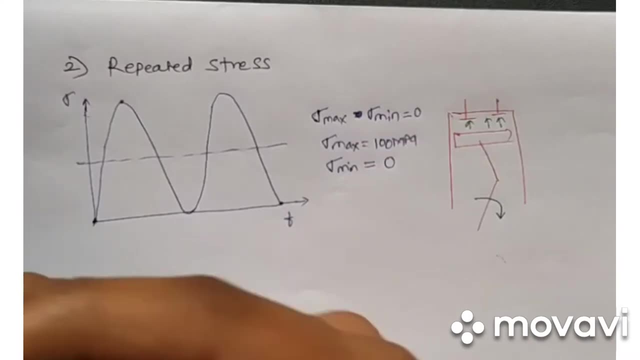 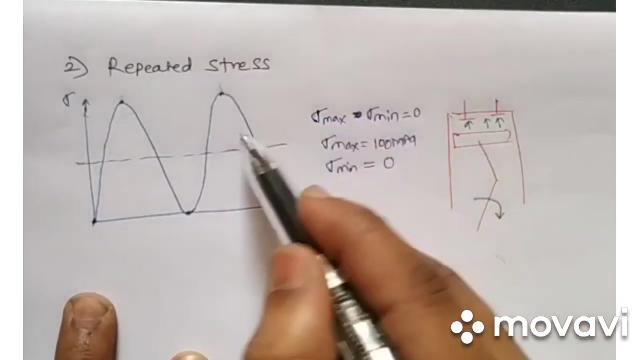 and again Sigma minimum will be zero. sorry, that means in the cycle the initial value will be something and after the period of time it is subjected to maximum value of stress. again it goes down, it becomes 0. then again, when there is a power stroke, it goes to maximum value of stress. 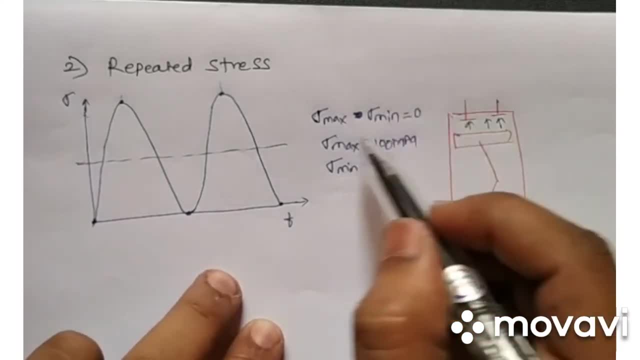 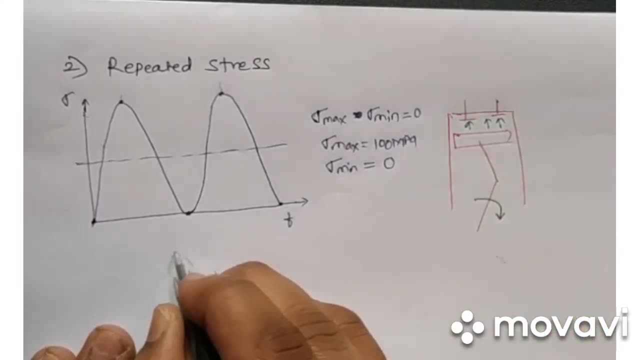 ok, so the minimum ㅁ value and the maximum value. okay, so we can write here now: Sigma mean will be my 100 minus 0 by 2, so that will be 50, sorry plus. then Sigma amplitude will be 100 minus 0 by 2. that will again be equal to 50, and we know R is Sigma. 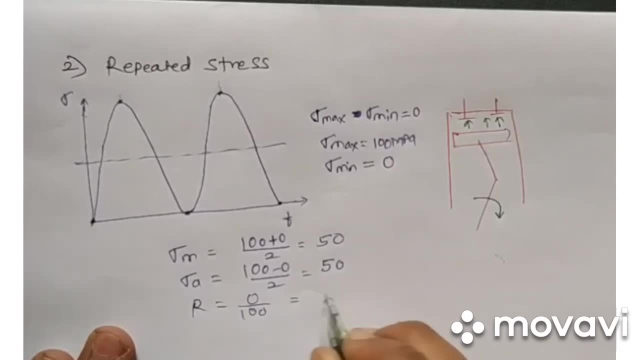 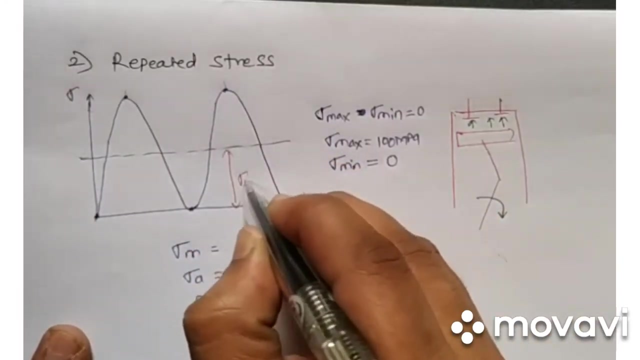 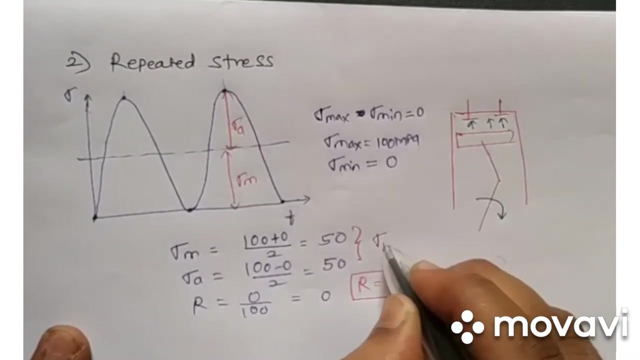 minimum by Sigma maximum, so this will be 0. so in this case the R value is equal to 0 in case of repeated stress, here we have a Sigma mean and here we have Sigma amplitude, and from this we can say that Sigma mean is equal to Sigma amplitude. 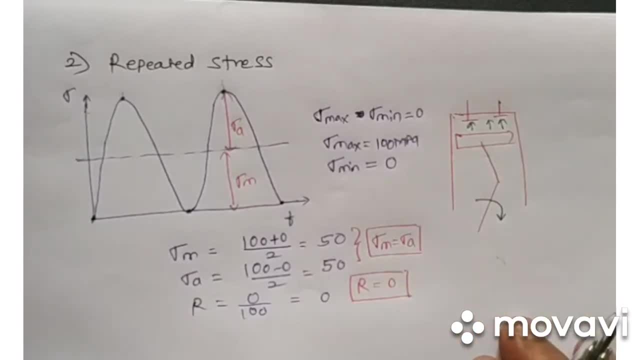 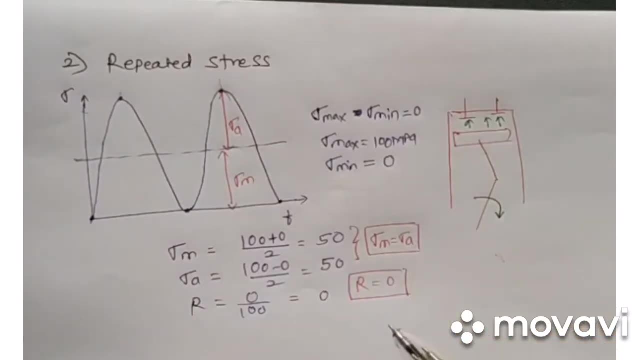 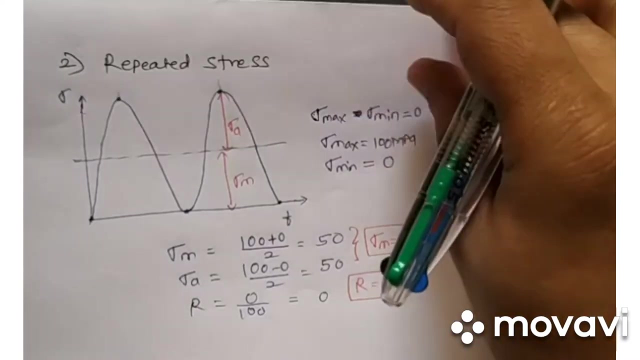 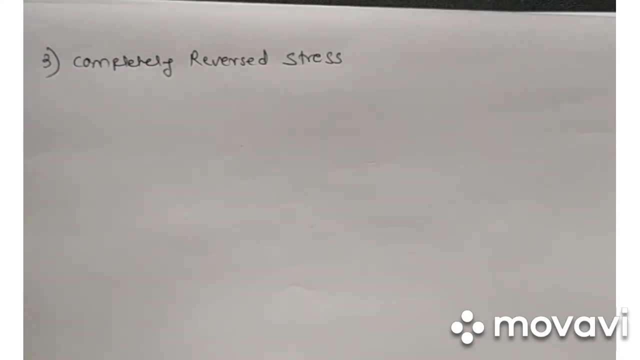 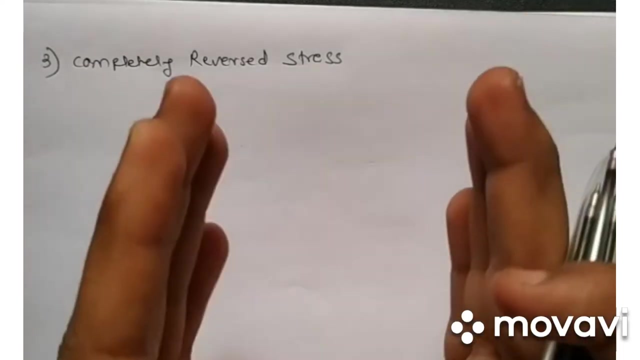 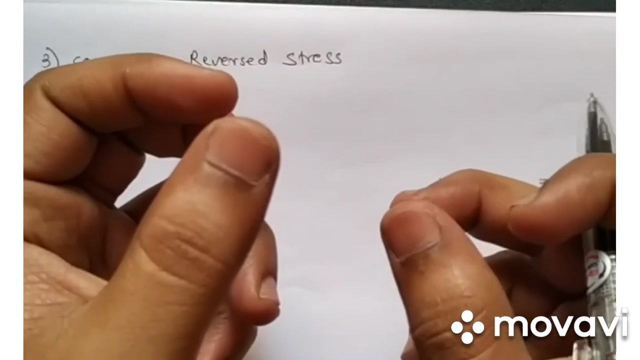 so this is another important thing. so, for a repeated stress, Sigma mean is equal to Sigma amplitude and stress ratio is 0. okay, now let's consider the third case, which is completely reversed stress. okay now, what does it mean? completely reversed stress? okay, so if at one moment there is a tensile loading, at another moment 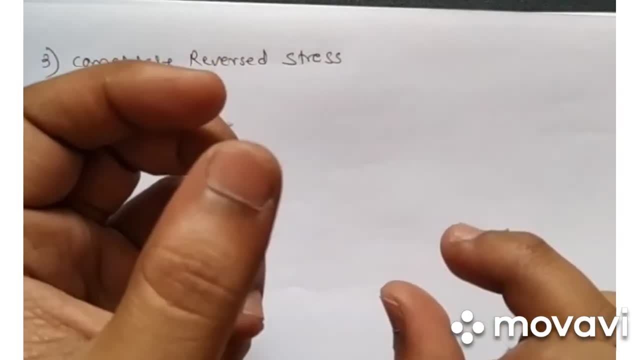 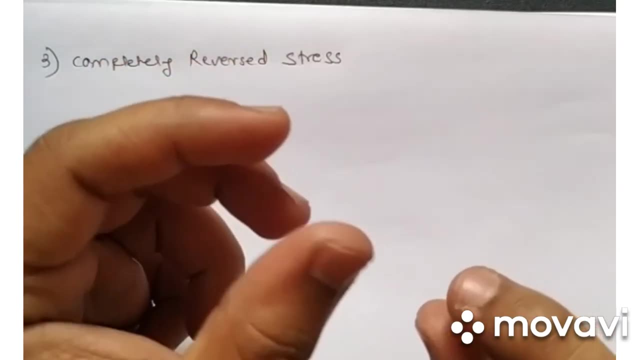 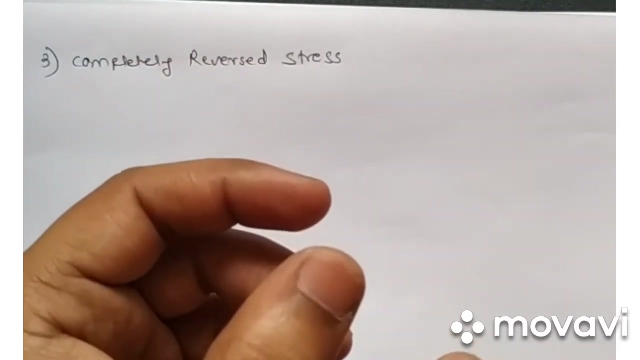 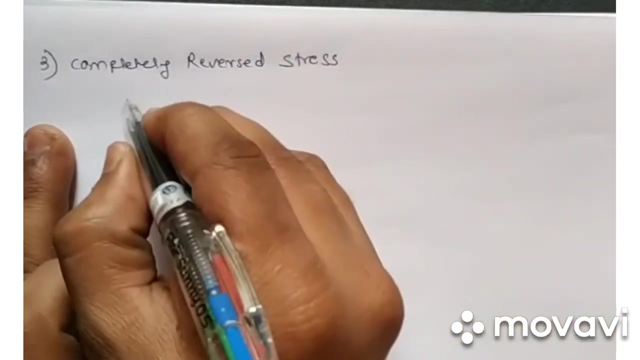 there is compressive loading of same magnitude but the direction is opposite. that means completely reversed one. I am rotating in this direction at another moment. I am rotating in this direction, but the magnitude of the stress is same. okay, so completely. in case of completely reversed the magnitude we 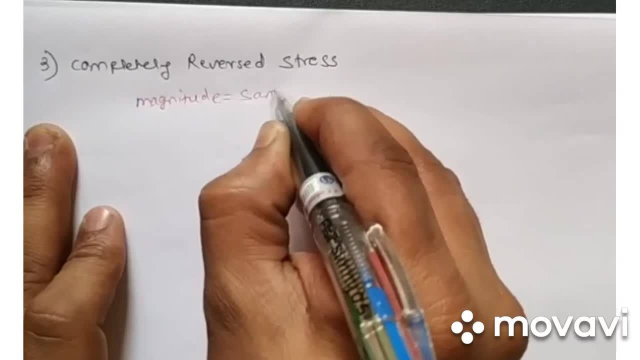 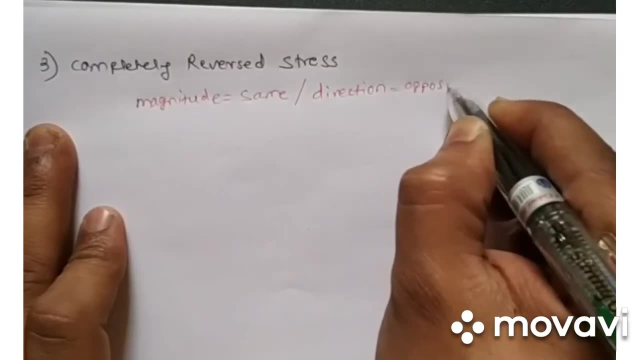 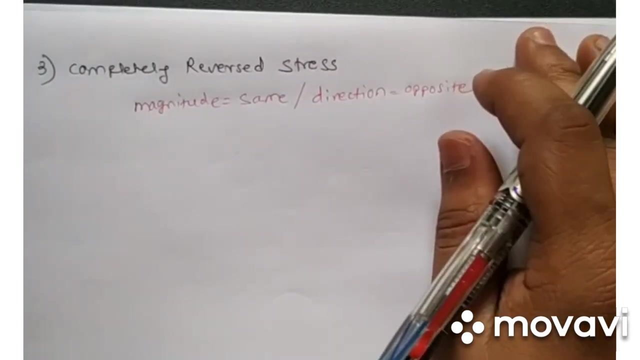 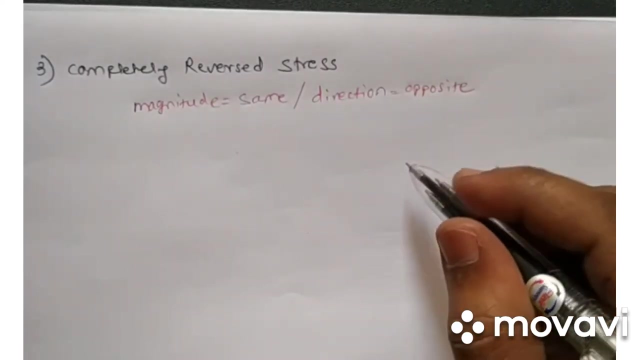 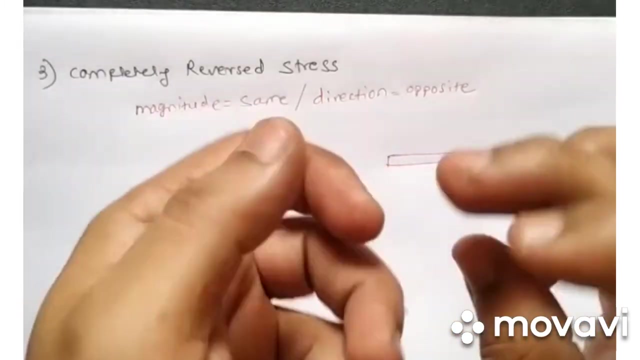 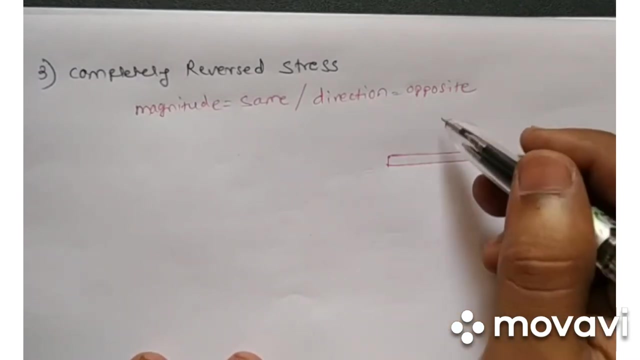 can say is same, but the direction is opposite. okay, so direction will be opposite. now we can consider the same example of twisting the, twisting the bar. or let's consider wire. so we are twisting like this, okay. so because of that, there are tensile stresses getting induced and 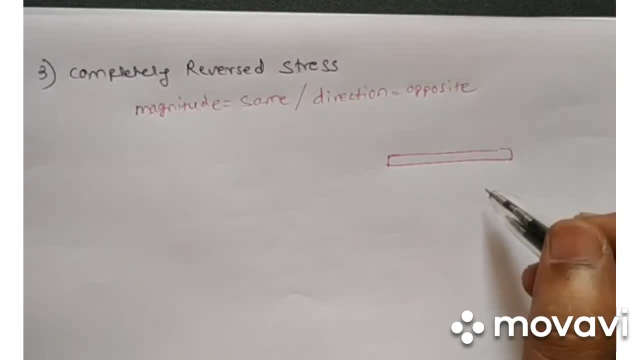 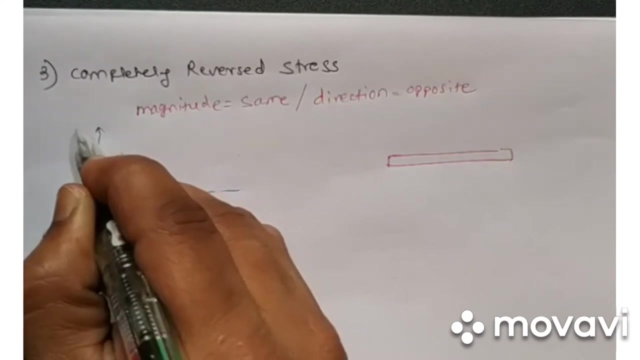 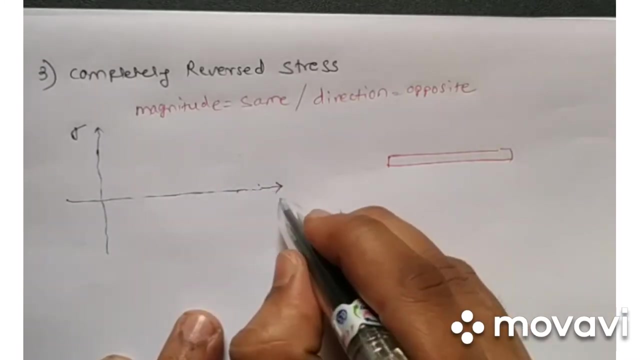 there are compressive stresses getting induced in the body and it is subjected to completely reversed stress. okay, now we will draw the graph for it and we will draw the graph for it. okay, so let's draw a graph for it. this will be our Sigma, this will be our T. okay, now what we can do here. first we will find out the values and then we will plot a graph, okay, so you can understand much more. so, likewise, here we said: the direction is opposite, but the magnitude is same. okay, so, um, my sigma max. okay, let's consider if it is 100 newton tensile, my 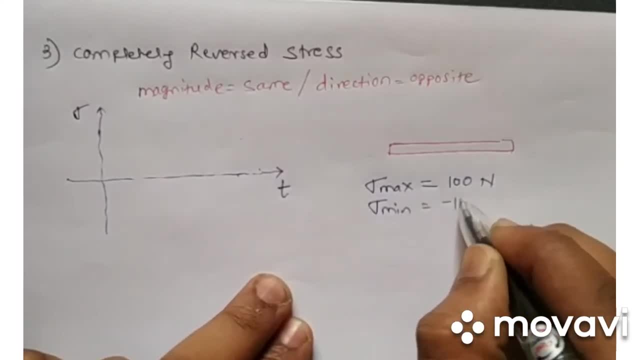 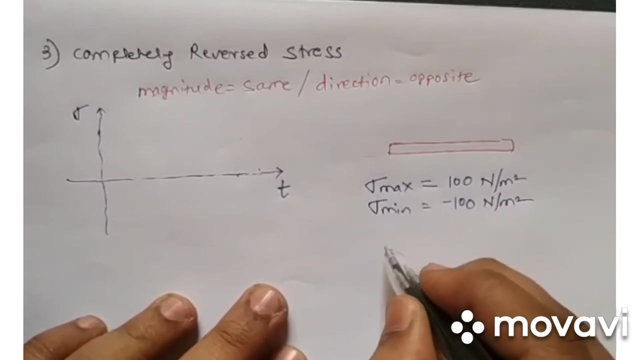 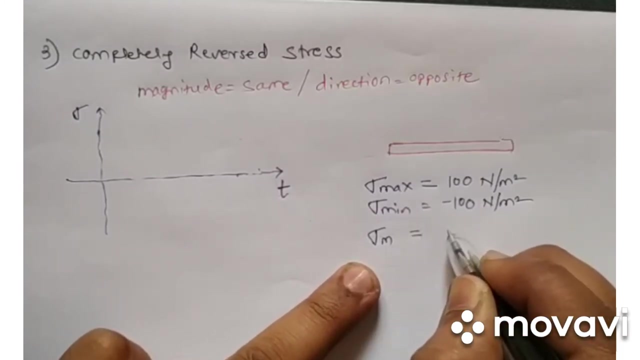 sigma minimum will be same magnitude, but the direction is opposite. okay, sorry, newton, per meter square. okay, so this is the meaning of completely reversed stress. so now we have the values so we can find out sigma mean. so sigma mean is sigma max plus, so this is minus by two. 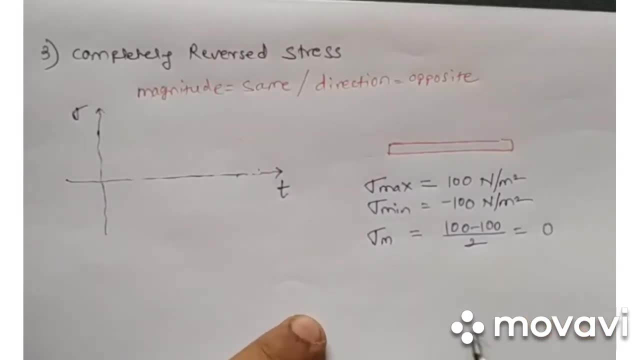 so this is equal to 0. and we have sigma amplitude, that will be hundred minus this minus hundred by two. so this be minus minus plus, this will be 100 mega Pascal, okay. and we have stress ratio, Sigma mean by Sigma max, so that is equal to minus 1, so here R is equal to. 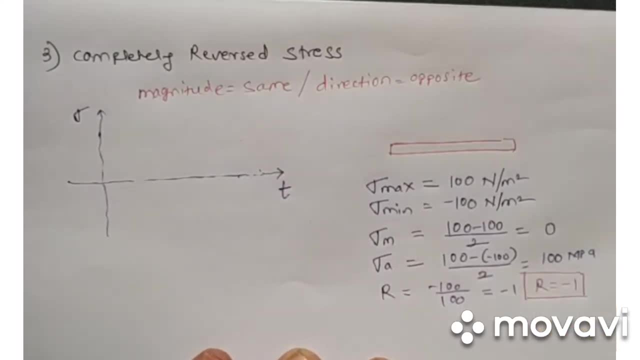 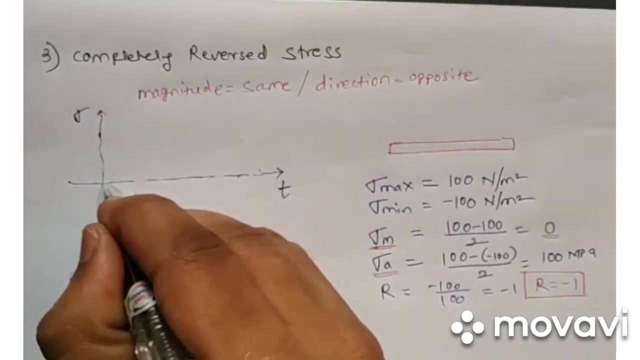 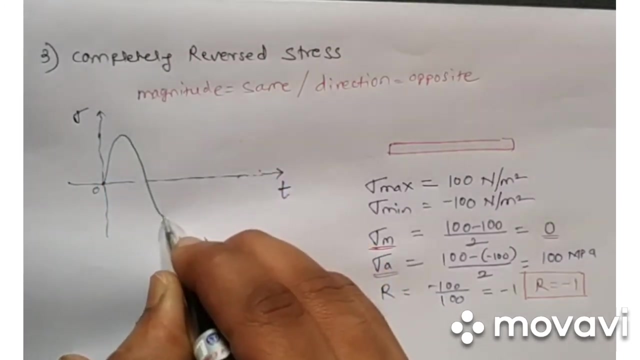 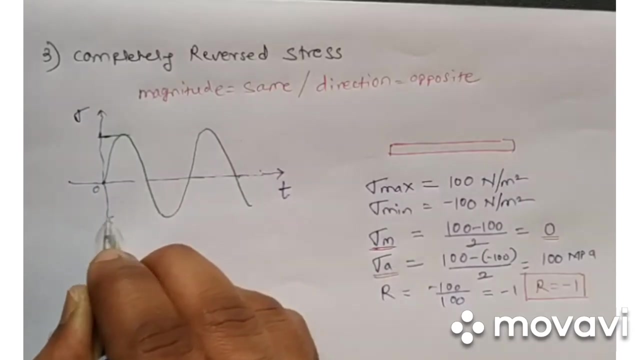 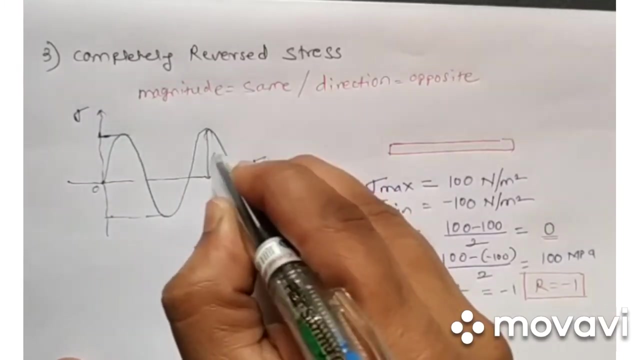 minus 1. okay, so we have Sigma mean at 0, okay, and Sigma amplitude is 100, which is same as Sigma maximum. so now we can draw the graph. this is 0, okay, so this is completely reversed. so this will be your Sigma mean, which is zero. this will be your Sigma amplitude. 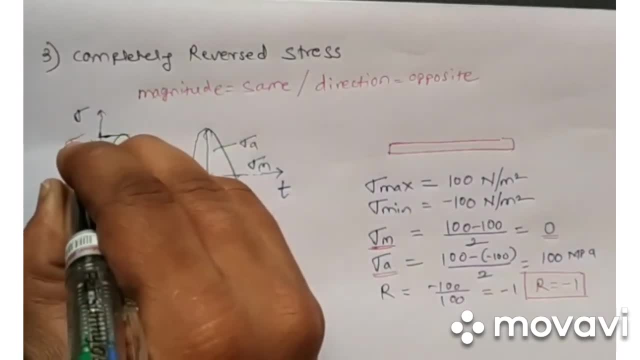 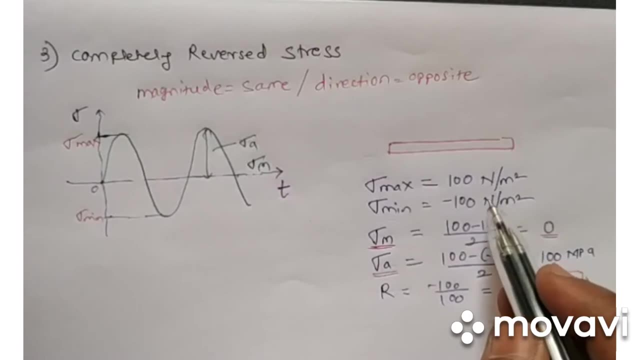 you have Sigma max here and here you have Sigma minimum. both will be same, like we have seen here, so both will be the same. that is Sigma maximum, skeleton, bottom, bottom. and last one: this is Gym she he. next one is: if you common forwards, this third cools in to one down. please stop flailing. we describe: 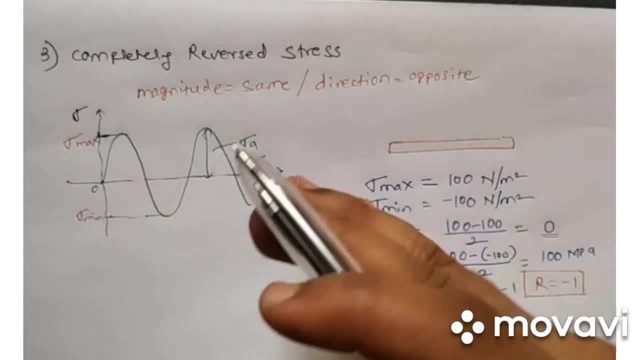 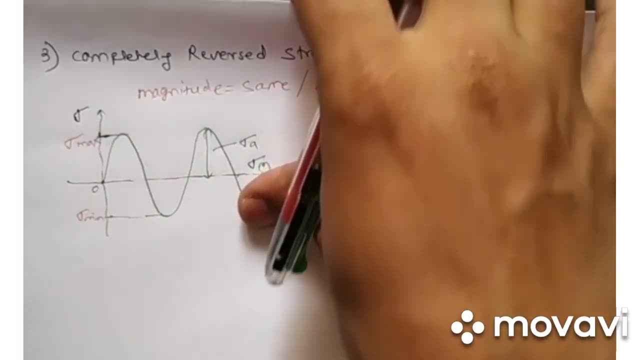 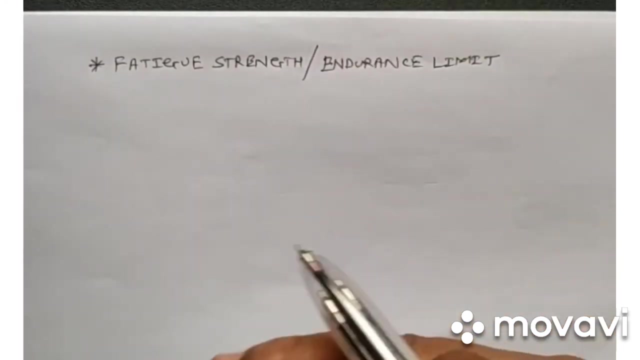 sigma. just Erica up because sigma is here. if your line here is equal to 1, which a and sigma minimum. so this is the condition of completely reversed stress. okay, now the important thing is how we can find out the fatigue strength or endurance limit of any material. so up till now we have seen what is the fatigue strength, what are the different loading? 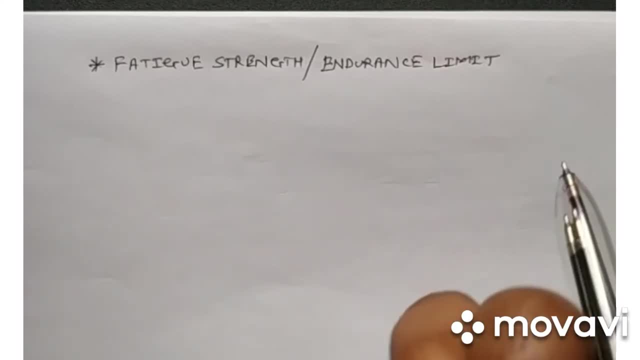 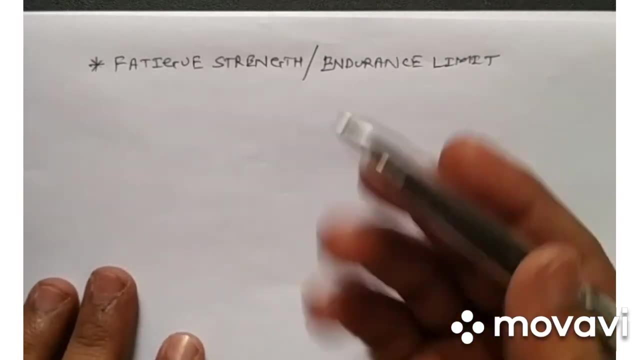 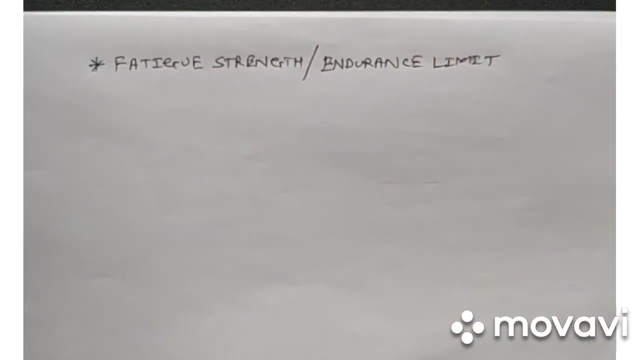 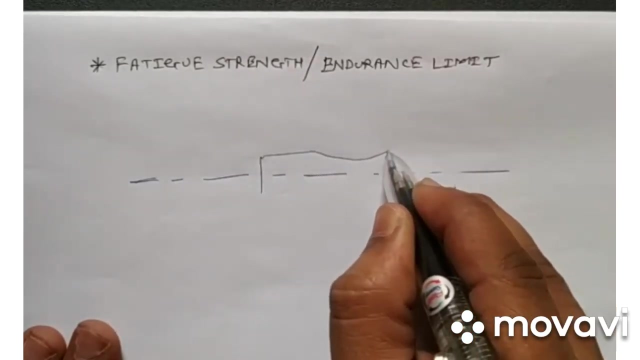 conditions and what are the different terminologies, so how this fatigue, strength or endurance limit is calculated. so, for that, we have a specimen and let's consider, for let's consider, steel material and we have a specimen with which is subjected to: okay, so so, so, so so. 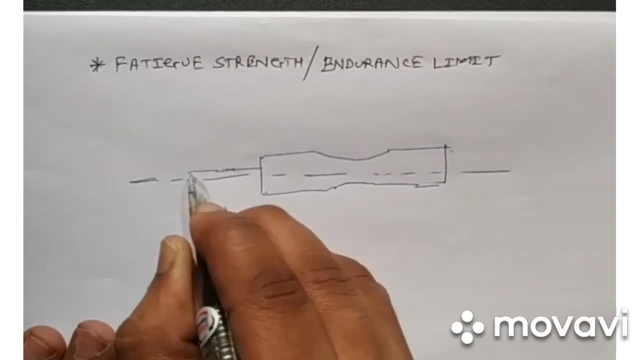 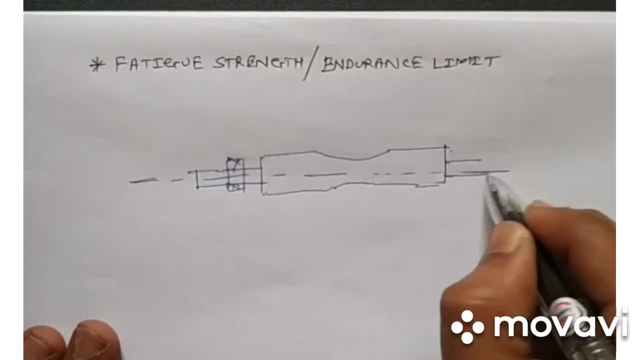 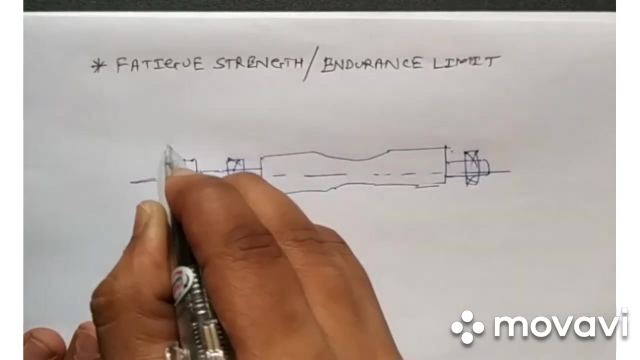 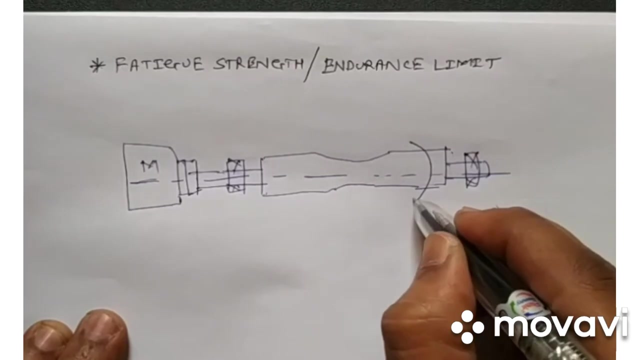 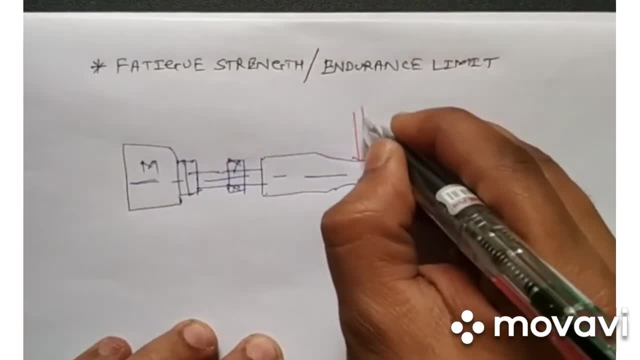 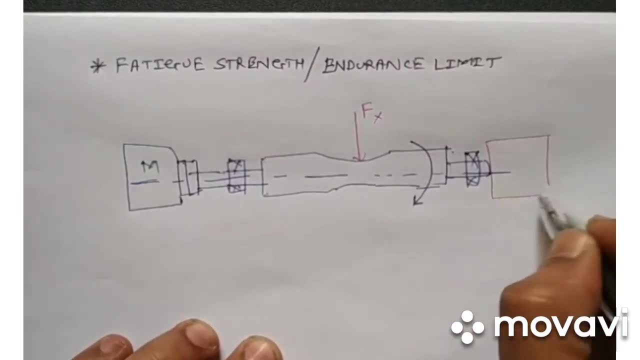 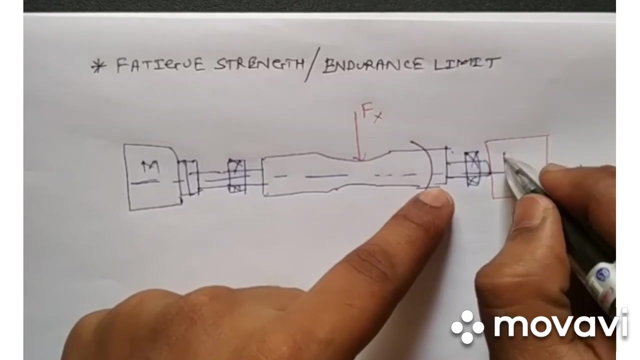 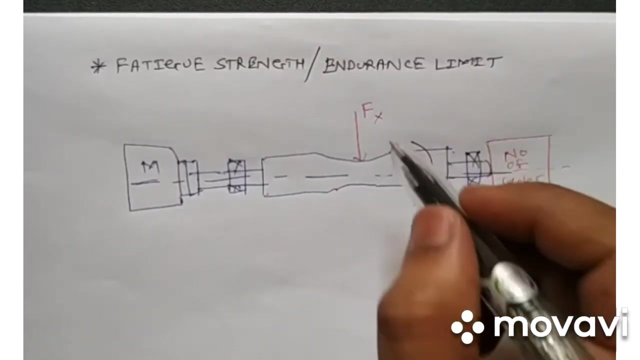 we are applying axial loading at the center, let's say fx, and here we have some provision to measure the rpm of the shaft. or we can say number of cycles. we are interested in number of cycles. okay, so this is the axial force which is applied on the shaft at the same time. this: 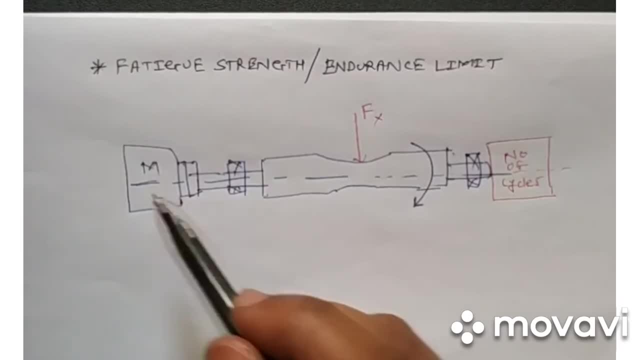 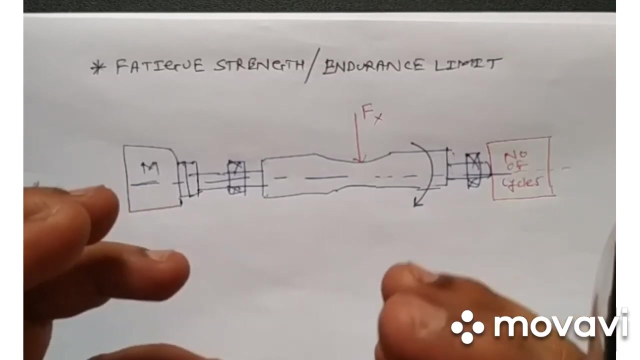 the shaft is subjected to rotation. that is the torsion. okay, now we have seen three different conditions. so what is this condition now here, if we see, this shaft is subjected to the load and it is rotating, so the shaft is subjected to completely reversed type of loading, and because of which 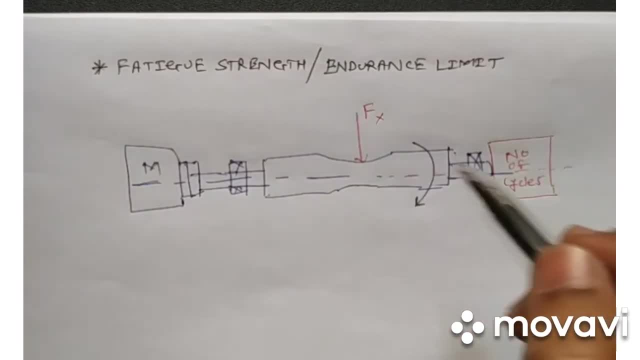 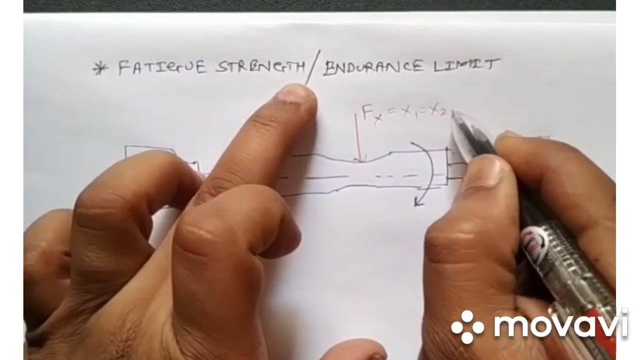 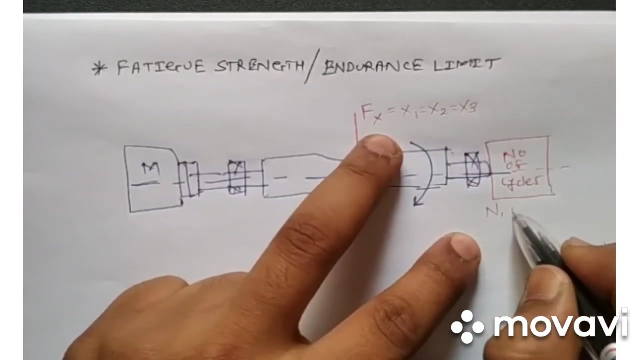 the completely reversed stresses generating and the shaft, and this shaft fails. now what we do? we apply some force initially, then we rotate the shaft and we see how much number of cycles this shaft can sustain before failure. then we go for x1, x2, x3, we go on increasing the value of this axial load and we get different n1. 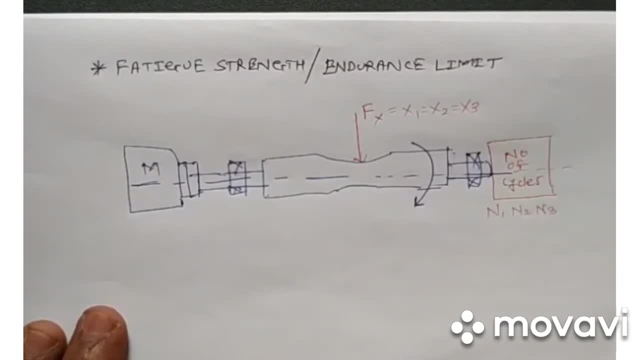 and 3. okay, that means, uh, we can write it into a chart. okay, so this will be your force and this will be your n. so, uh, we have x1, x2, x3 and corresponding n1, n2, n3. now it is a, it is. 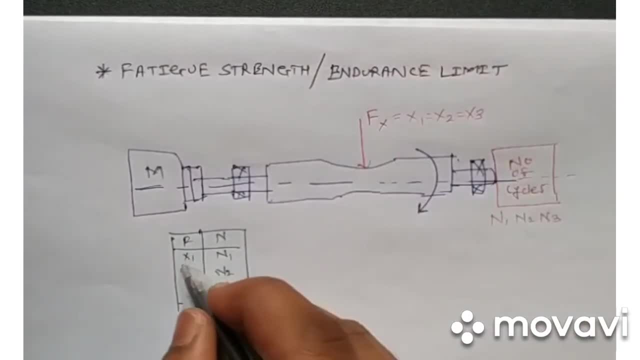 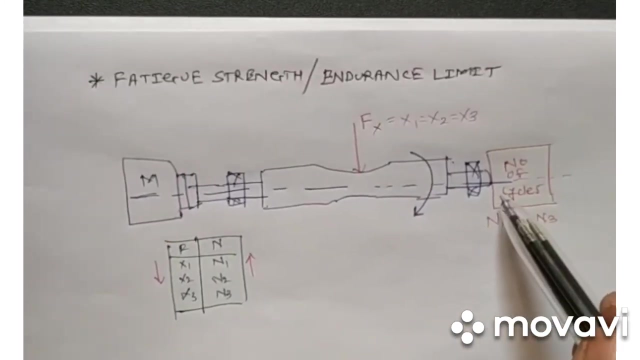 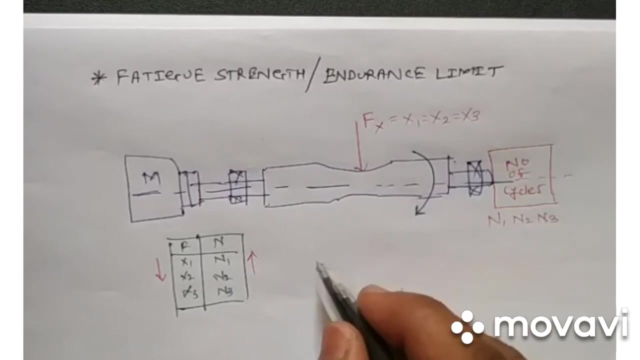 you know obvious that i am. when i am going to increase the load, this n value reduces. what does it mean? that if i am going to increase this f value, the number of cycle at which the shaft is getting failed is reducing. okay, and from this data we plot a graph which is called as sn curve. 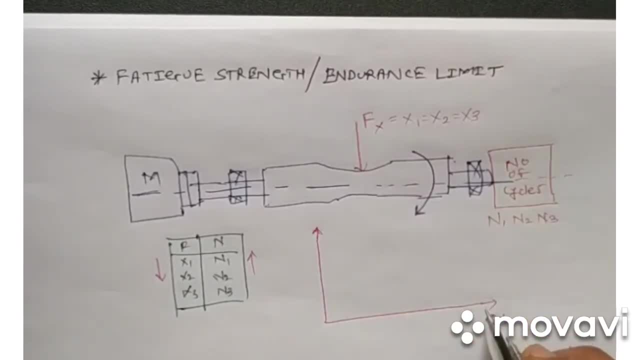 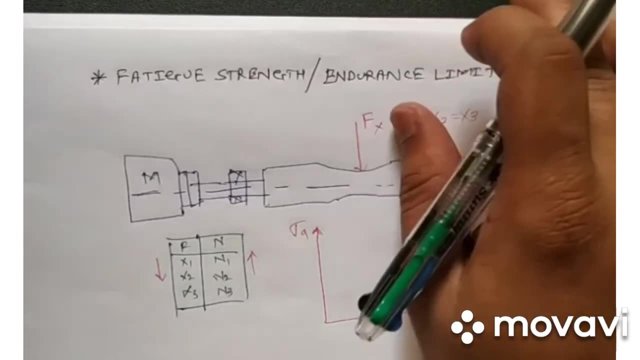 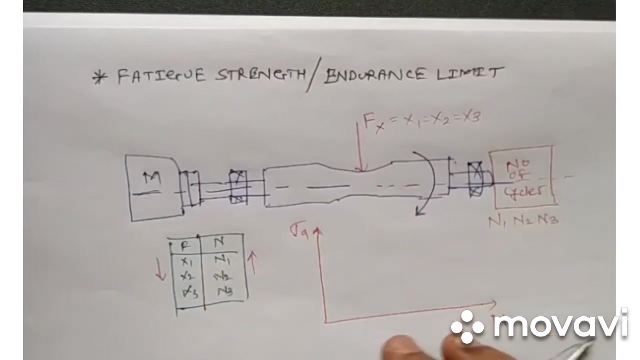 which is nothing but n. we have here n number of cycles and here we have sigma amplitude. so this is called as the sn curve. we will see it into the details. so graph is plotted from these values and is called as sn curve. that is nothing but stress into number of cycles. 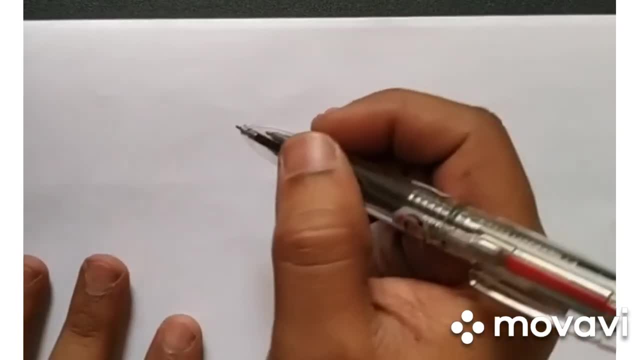 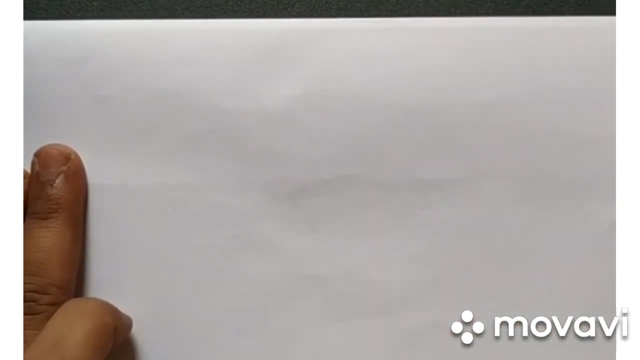 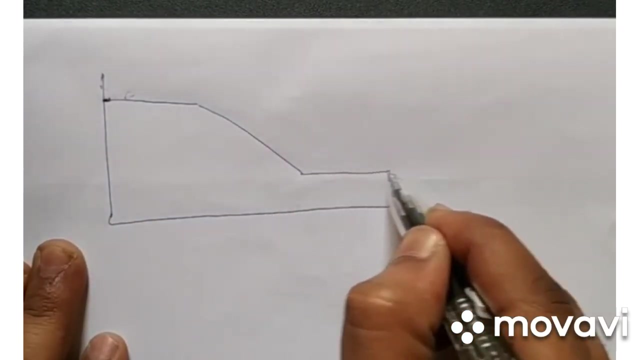 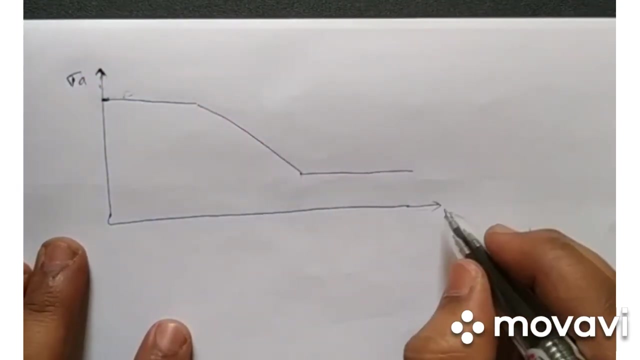 okay, so from the data which we have obtained, uh, we draw a graph. okay, so the graph will be like: oh, this will be an. this is your sigma amplitude. okay, and this is your 种 계標ie. Building log n test. drop thousandwald a great often. 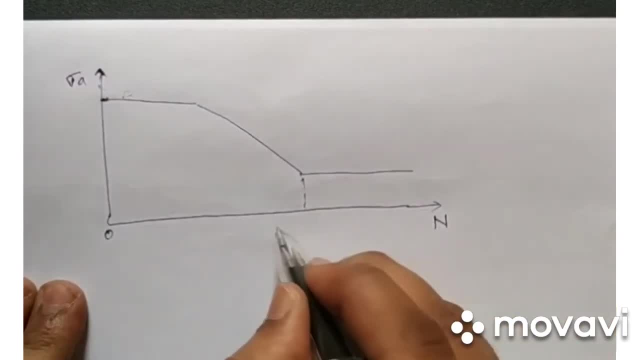 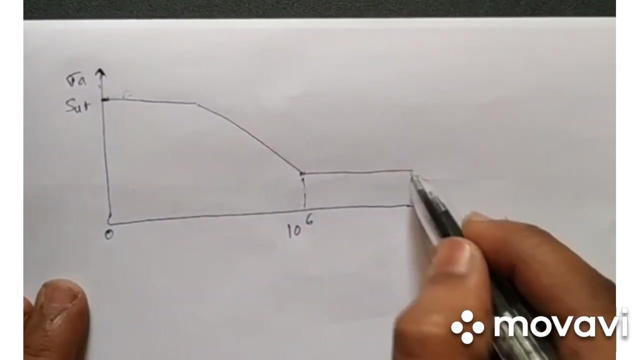 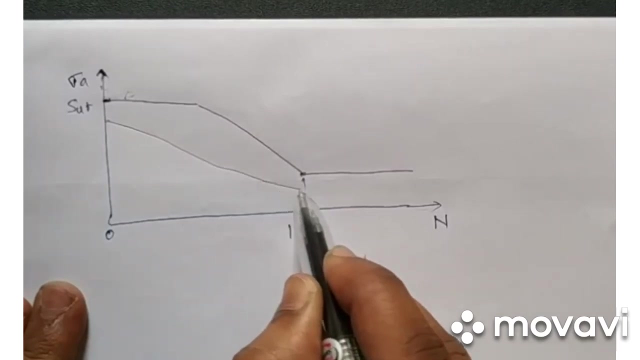 number of cycles. let's say this is zero, let's say this is changes to six. okay, this is your su, the ultimate strength, and you will be having the endurance strength of the material. and let's say: this graph is for steel, for aluminium, the graph will be different one. let's say: okay, 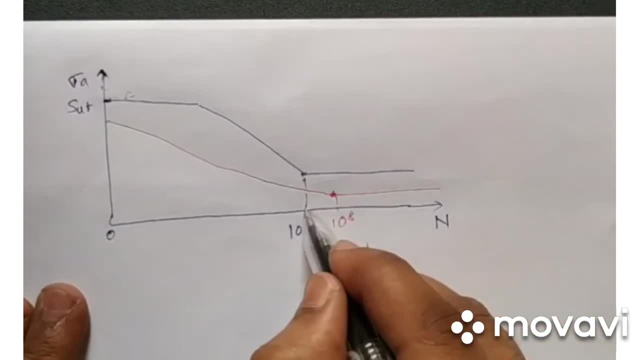 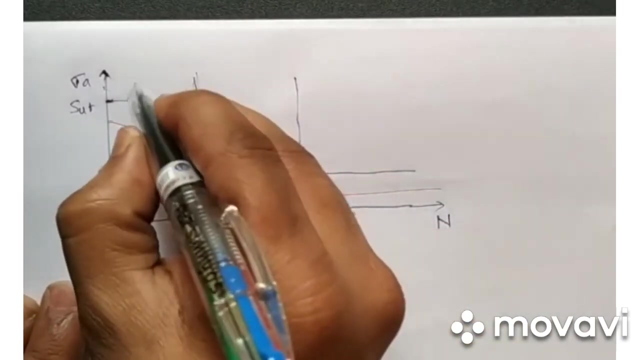 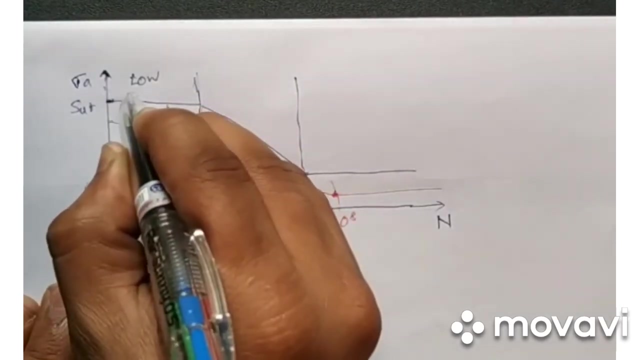 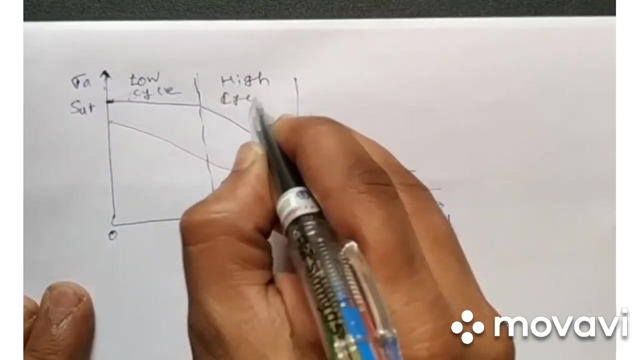 so this is tenders to eight and this is 10 s to 6. so for different materials, again, this graph will be different. and if we will divide this graph into bars, so this is called as low cycles, no fatigue cycle, these are high fatigue cycle and these are 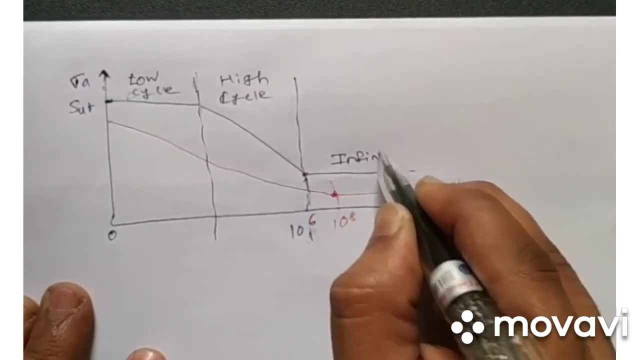 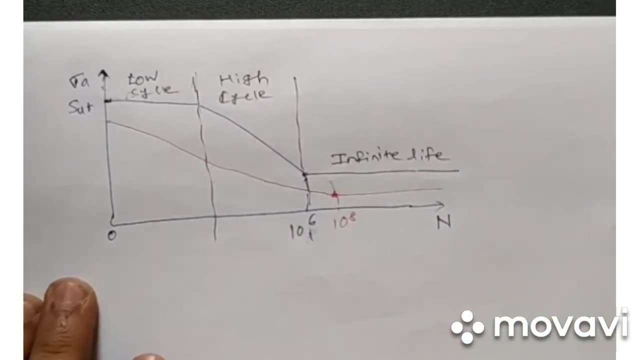 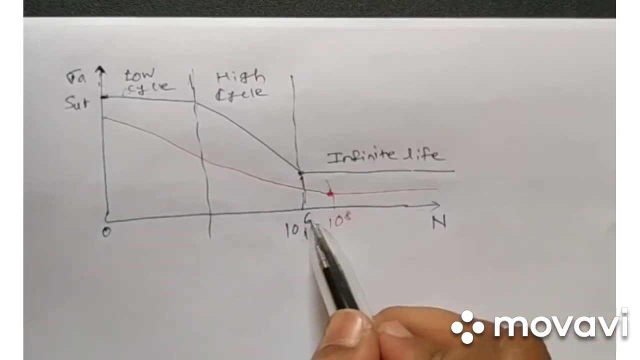 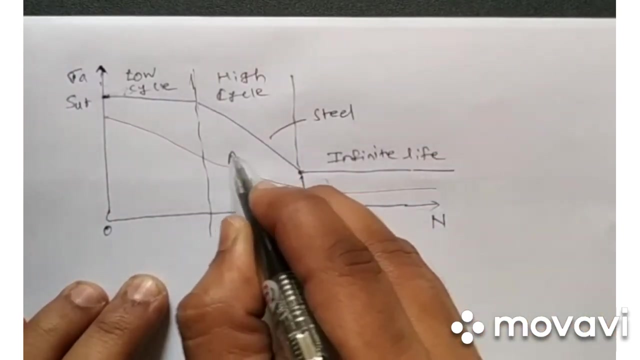 infinite life. okay, this is low cycle. then this is low cycle fatigue design, this is a high cycle fatigue region and this is the infinite life. okay, for the material. now we can see this graph becomes asymptotic. that means it becomes horizontal at 10 raise to 6 cycles for steel. so this is for steel and this is for aluminium. so for 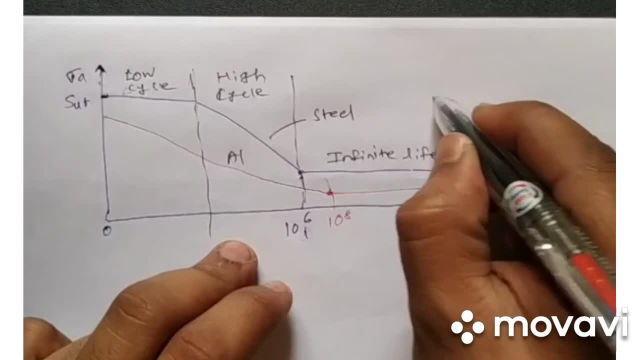 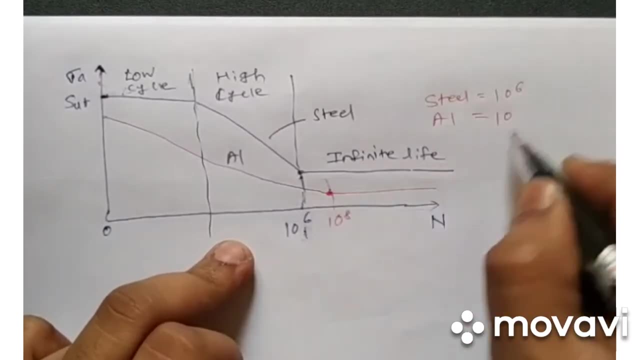 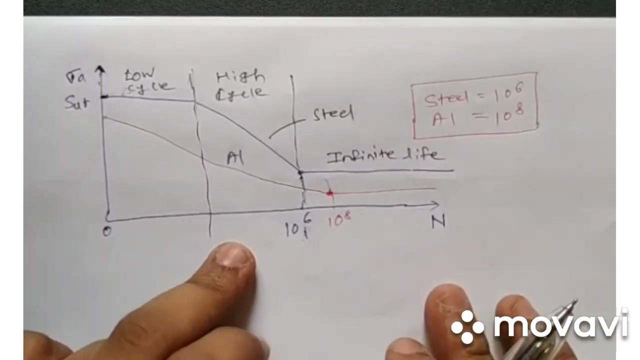 steel, this graph becomes asymptotic at 10 raise to 6 cycles. and for aluminium, it becomes asymptotic at 10 raise to 8 cycles. okay, so endurance strength- what exactly it is? that is nothing but the maximum stress amplitude which a standard specimen can withstand for a minimum. 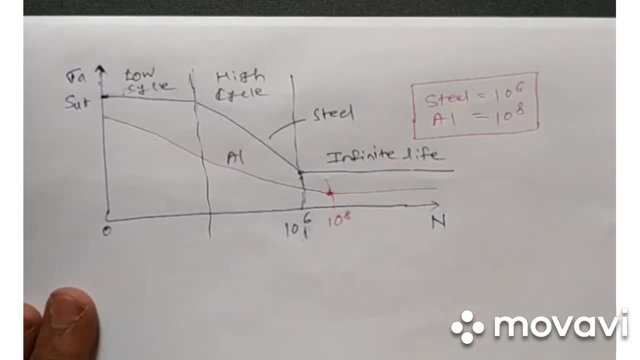 life of 10 raise to 6, that is, 1 million revolutions under completely reversed loading condition. okay, we subjected that part to completely reverse loading. so the value of stress that the material can withstand for a minimum life of 1 million revolution under this loading, that is nothing but the endurance limit. 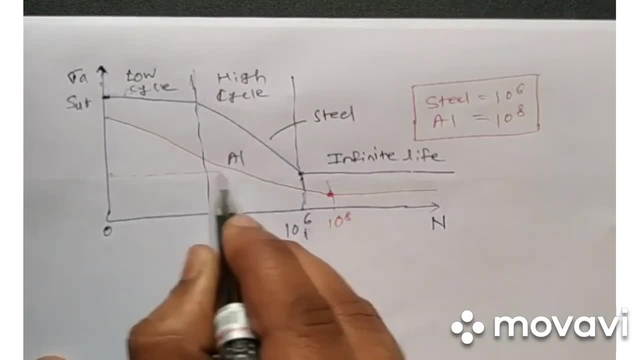 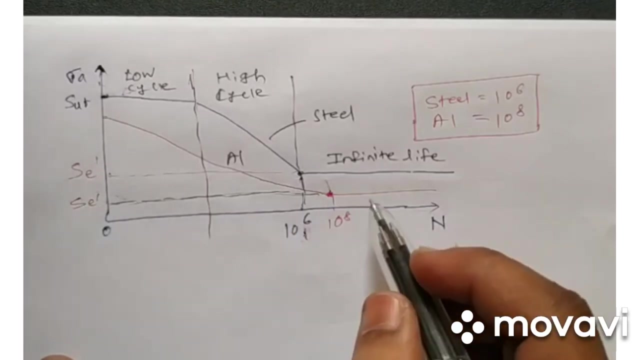 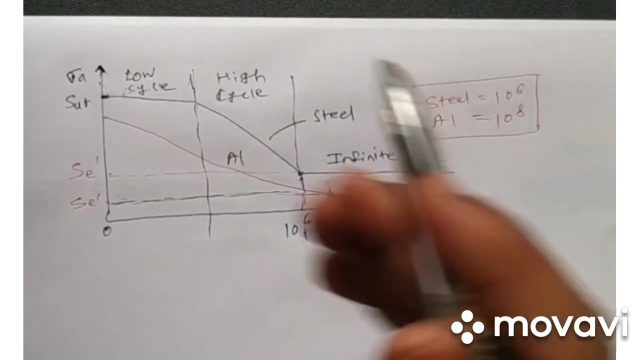 which is also denoted by, let's say, this is is se dash. i will say what it is. therefore: aluminum, it will be se dash. this is for aluminum, okay, and this is for steel. so that is our endurance limit. now, this endurance limit, we have a low cycle, we have a high cycle and we have an infinite cycle now where we have to design. 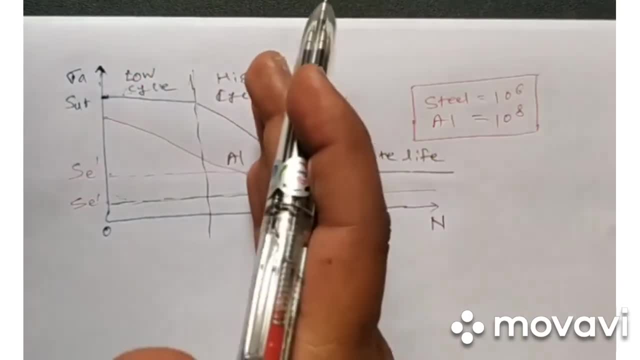 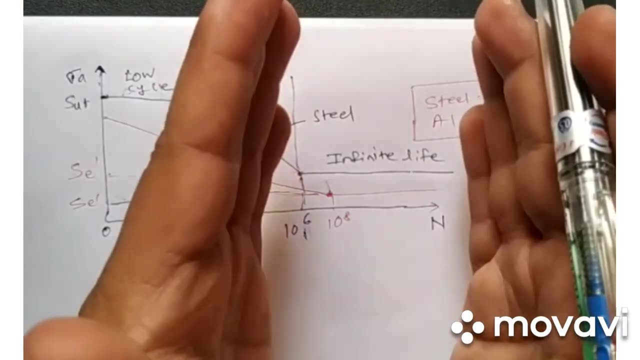 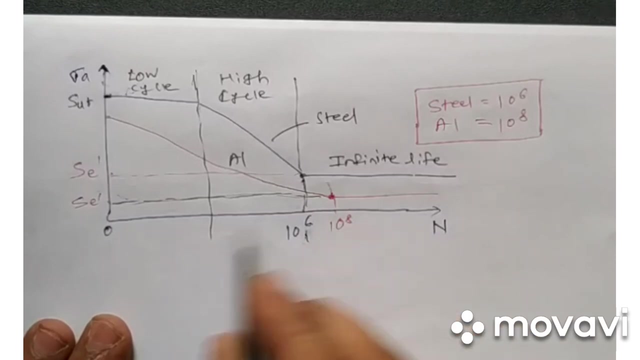 the material for low cycle fatigue life, high cycle fatigue life or infinite life. this is also important. we can't design all the materials or all the designs in this infinite life. let's consider one example: if, if you take a, if you take a matchstick, and if you design it for infinite life, then what will happen? 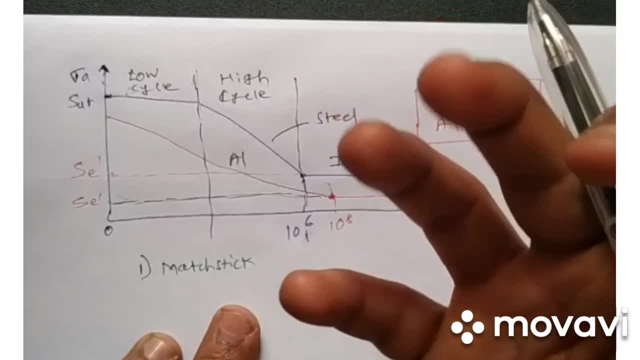 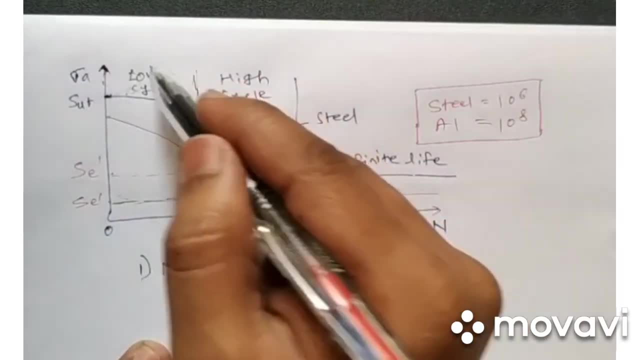 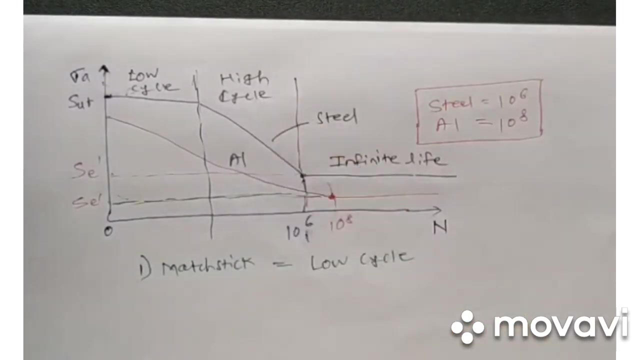 if you rub it it will not get ignite. but what we want? we want to ignite the matchstick as early as possible, so we have to design it for the low cycle. so matchstick is designed for low cycle. now let's consider high cycle. okay, now let's consider a pressure cooker. 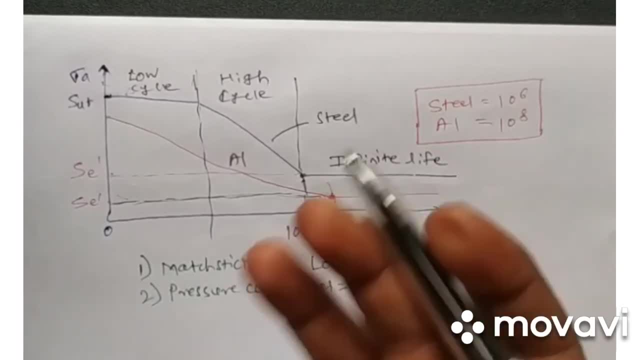 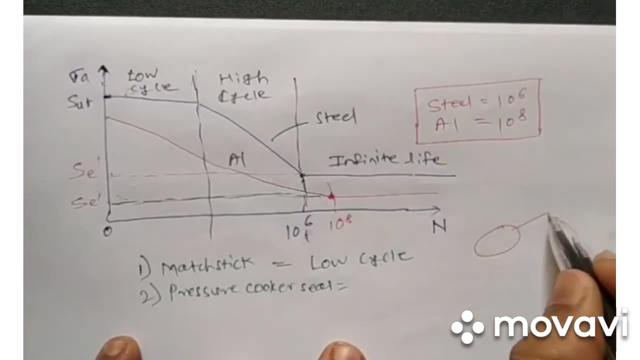 cooker c. now, i don't know how many of you have observed, uh, in a pressure cooker, that is the top plate of the pressure cooker- you have one seal here, okay, and this seal explodes when the pressure inside the bowl becomes greater than the value for which this seal is designed. now, this pressure cooker is importantly. if it burns, it can harm the 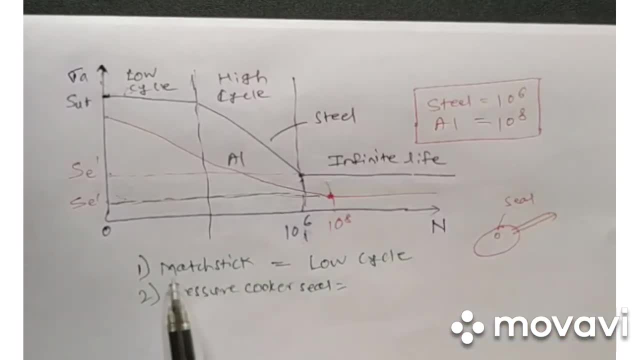 people, so it shouldn't move before we just open theacaksın. but i have to drill. it' get failed at much earlier life, so we can't design it for this low cycle, but at some value it should get failed also. otherwise what will happen if it doesn't fail? it can cause a harm, so we design this. 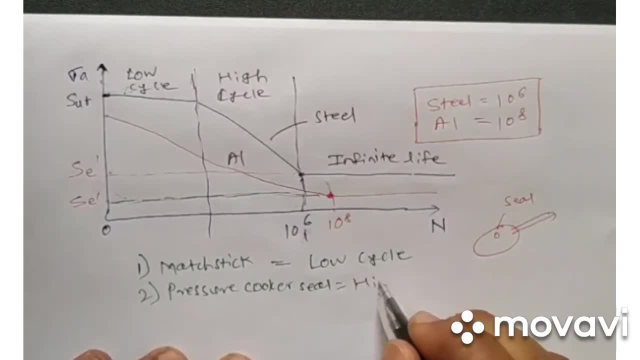 pressure cooker seal for high fatigue. cycle life, and next is the infinite life. so infinite life, let's say a bearing for a bearing. it is very important that it should not fail earlier. it has to run for longer and longer. so here our main aim is that the bearing should not fail. 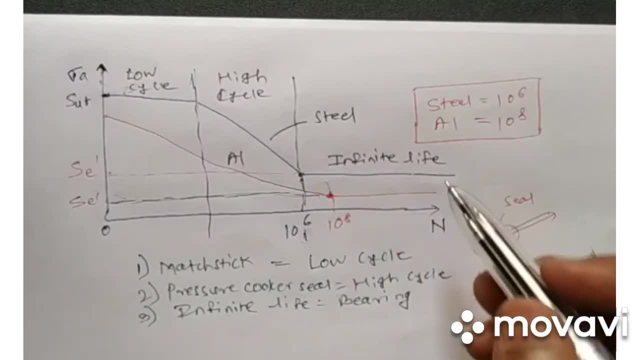 so we have to design it for the infinite life. so it is very important that which zone you are picking for the designing. it is not like you should always design so that the material shouldn't fail like in like. we have considered the example of matchstick. so this is very important and 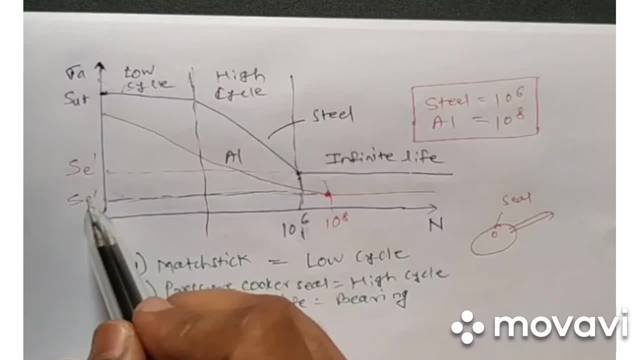 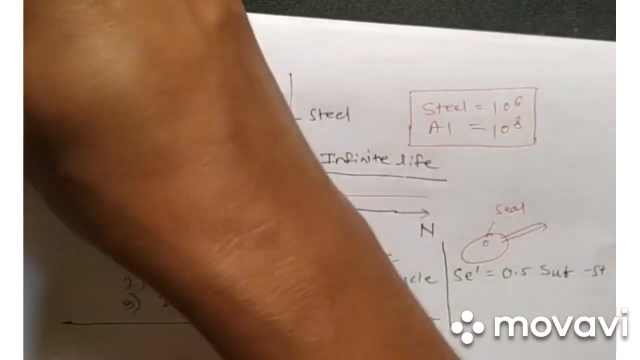 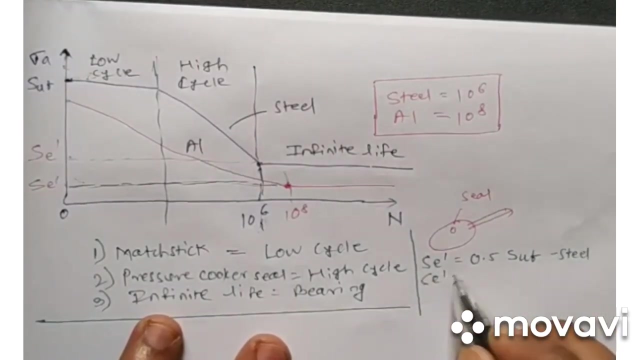 this endurance strength depends, uh, on so many different factors, and there are standard relations like this: s? e dash is equal to 0.5 times of s? u t for steel. okay, so for steel, uh, it is, uh, it is uh 0.5 times. then uh, for cast iron, it is uh 0.4 times. and